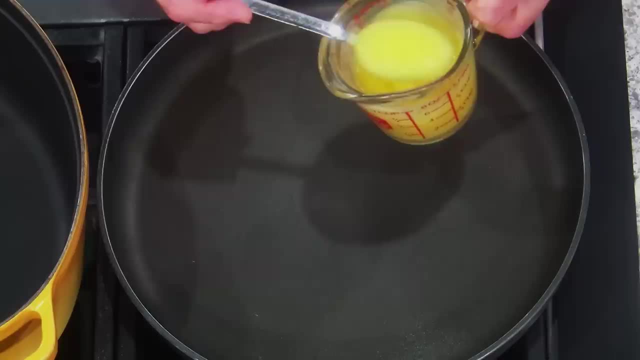 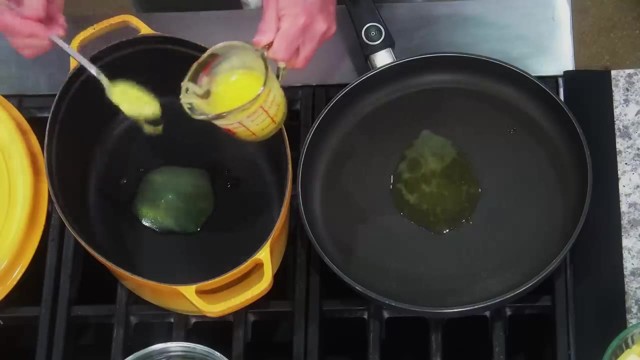 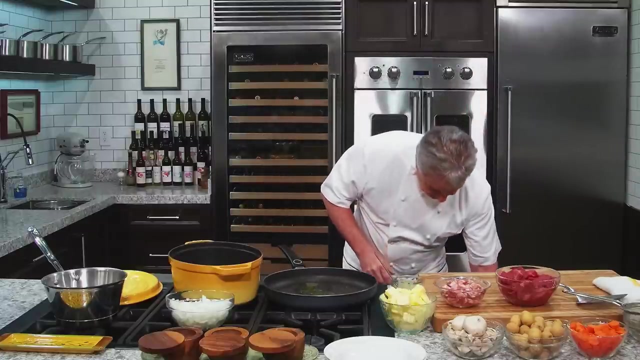 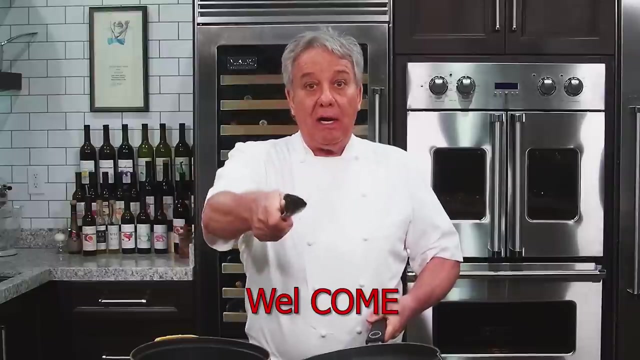 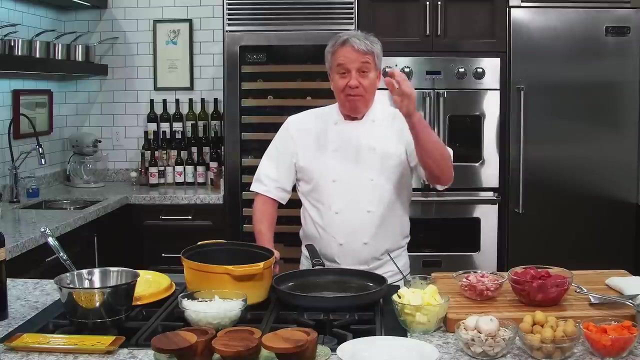 We have a little mise en place, But before I get going, I'm going to saute a little bacon And I'm going to put a little butter in there. You don't really need butter to put, But I got clarified butter right there, friends, And this will work. The reason why I use clarified butter is because it doesn't burn as much as regular butter. You know that right. Of course, you know that You've been watching my channel. For all of the new people that have never watched the channel, welcome to the coolest cooking channel on YouTube. Thank you for watching and thank you for subscribing. We've had so many great subscribers. You guys are amazing. 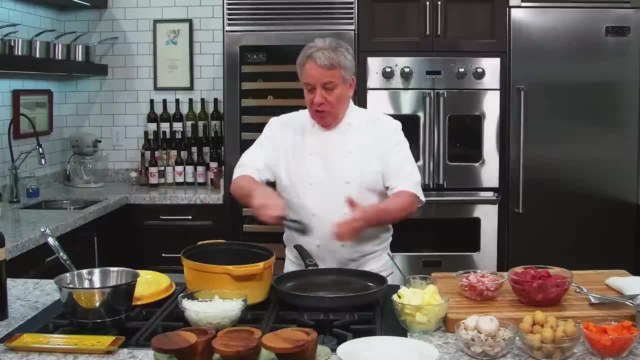 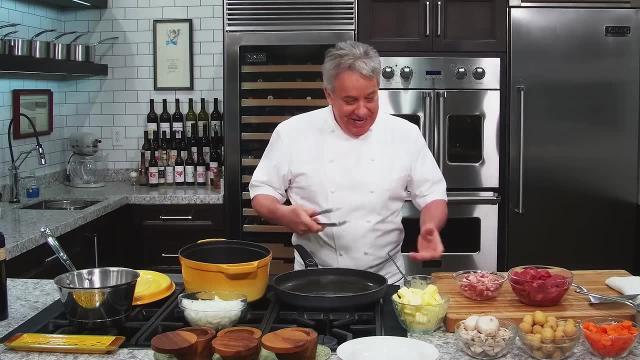 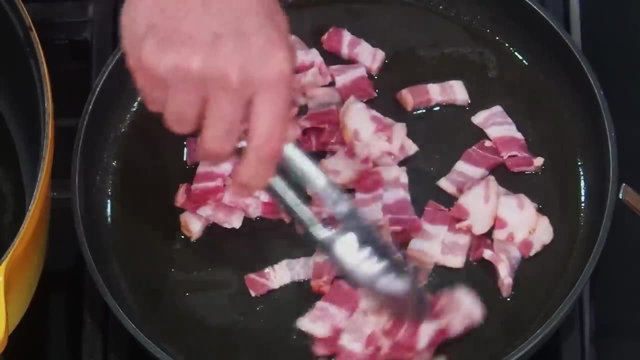 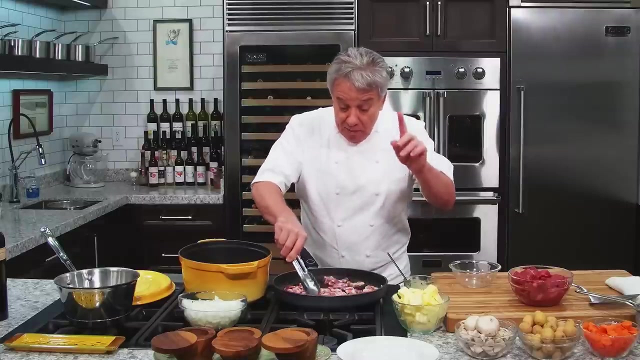 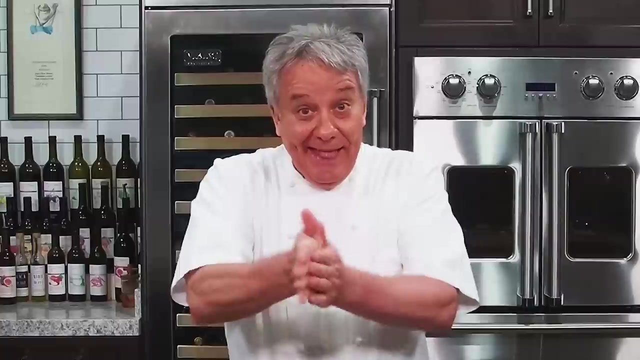 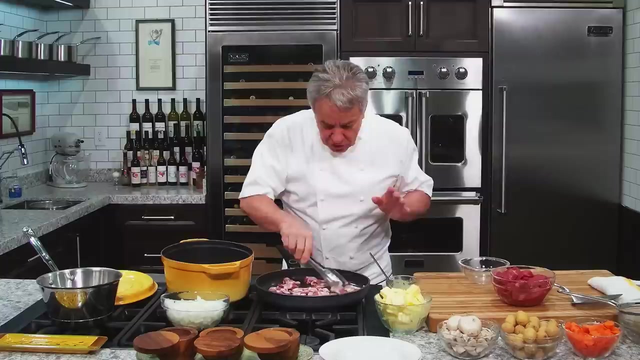 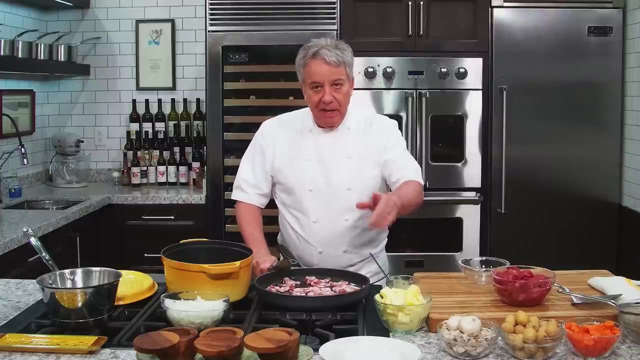 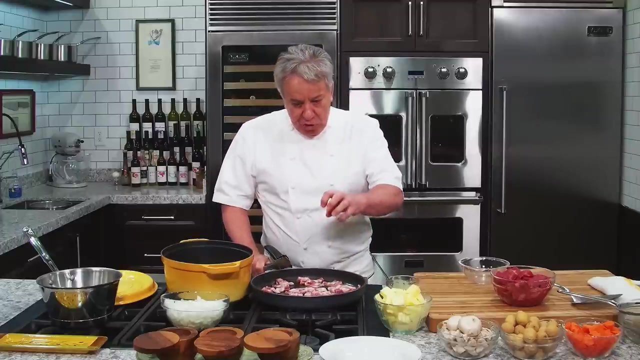 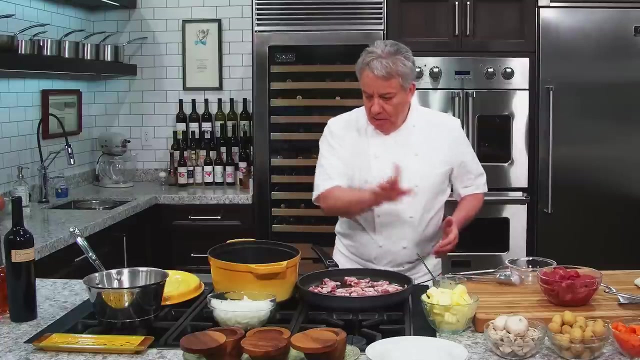 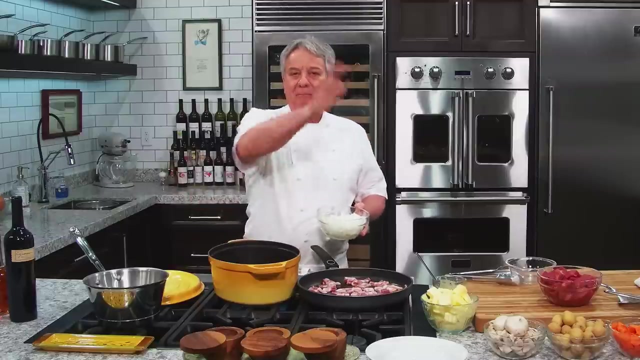 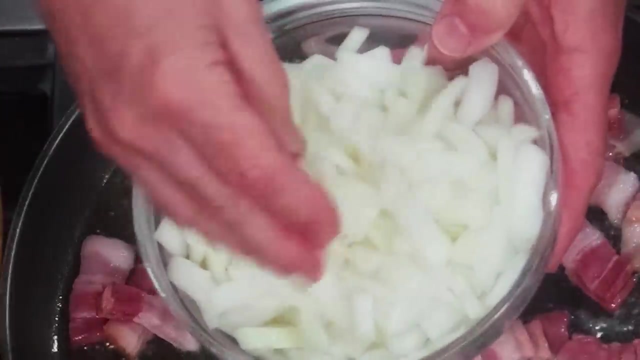 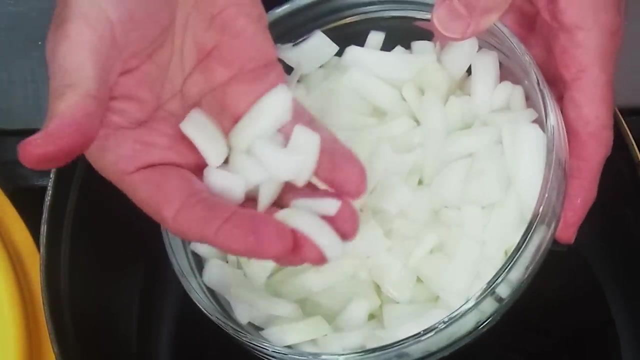 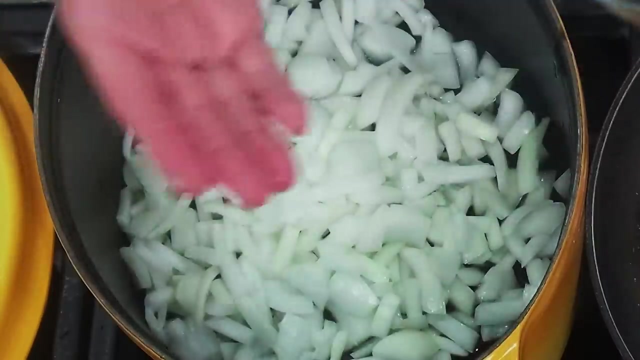 Thank you for watching and thank you for subscribing. We've had so many great subscribers. You guys are amazing. Thank you for watching and thank you for subscribing. We've had so many great subscribers. You guys are amazing. Thank you for watching and thank you for subscribing. You guys are amazing. 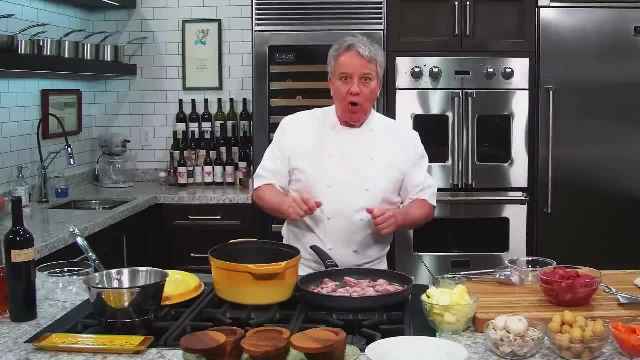 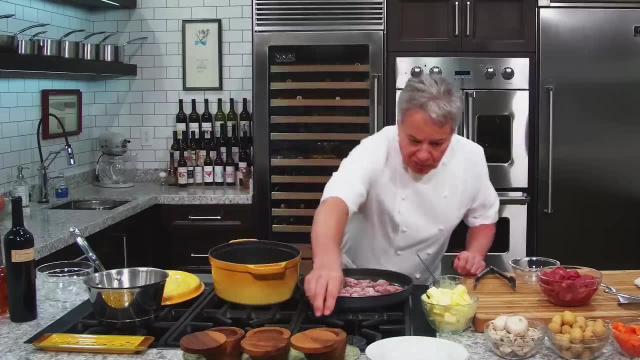 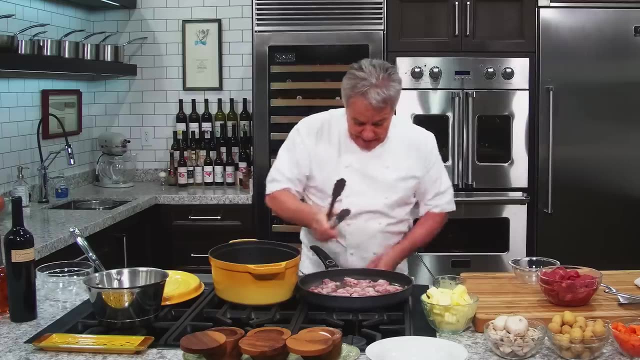 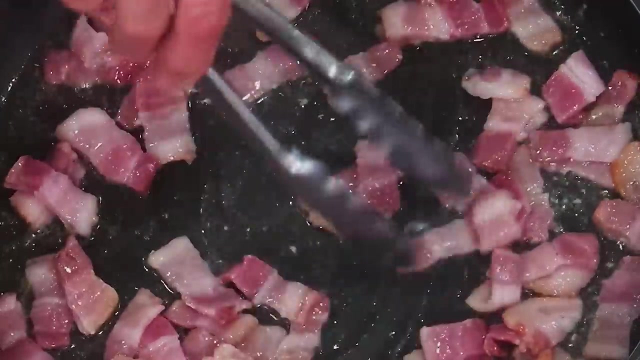 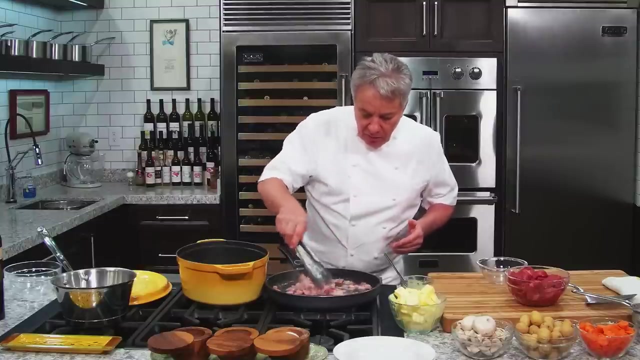 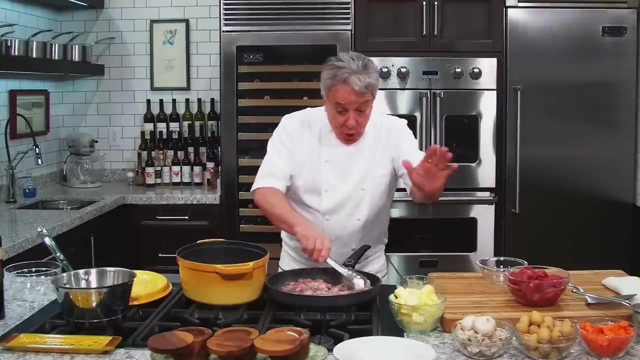 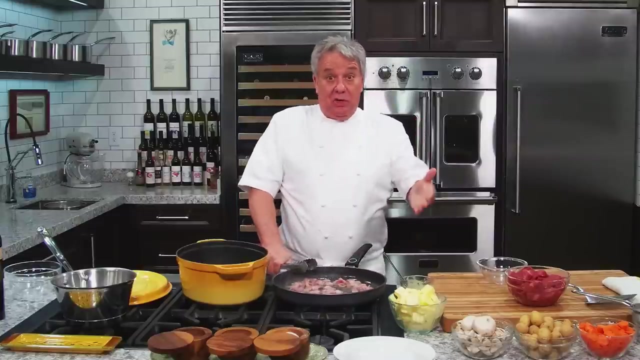 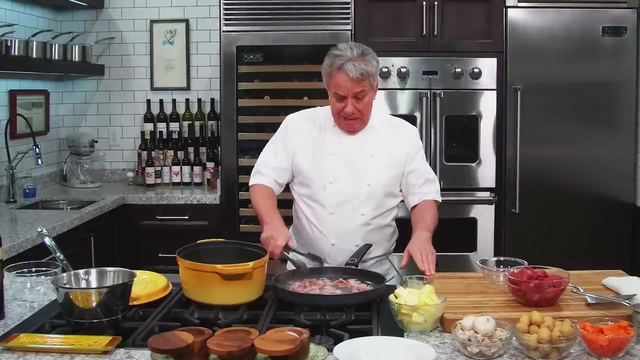 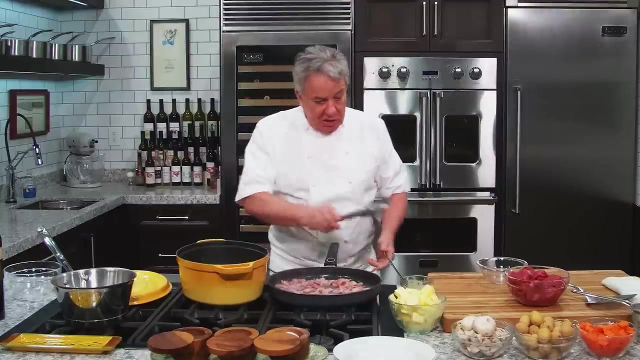 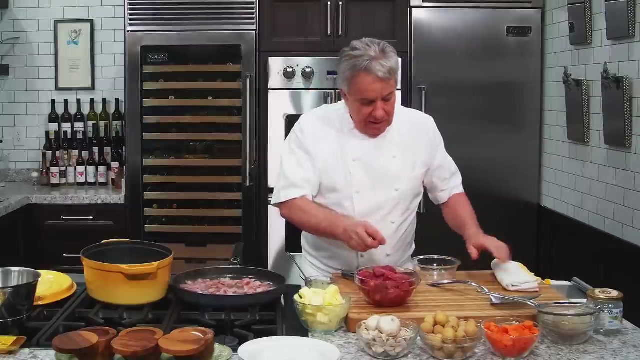 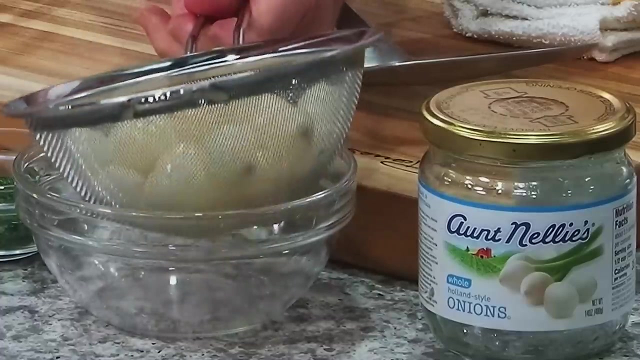 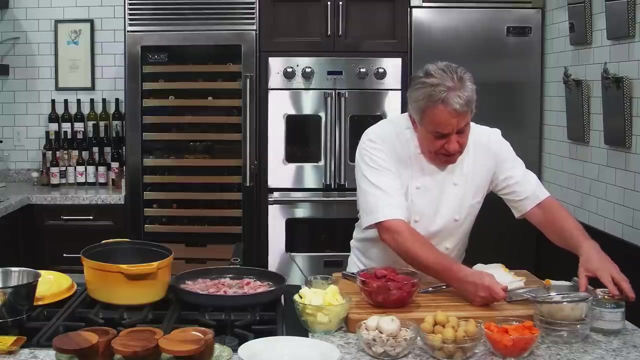 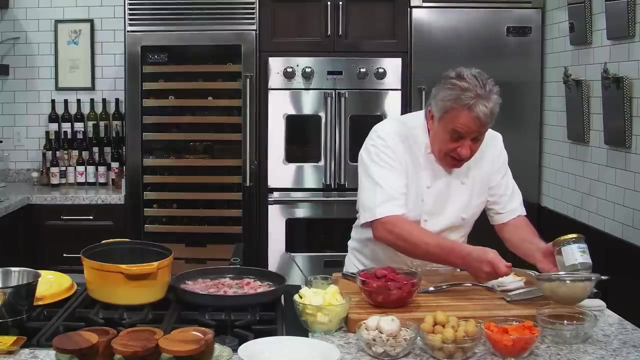 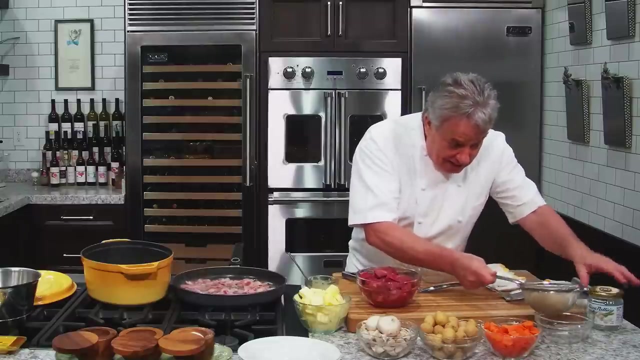 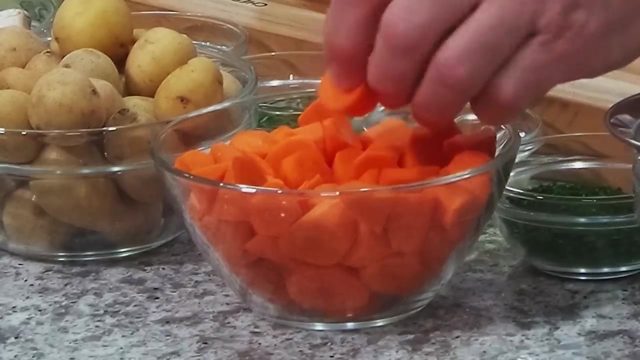 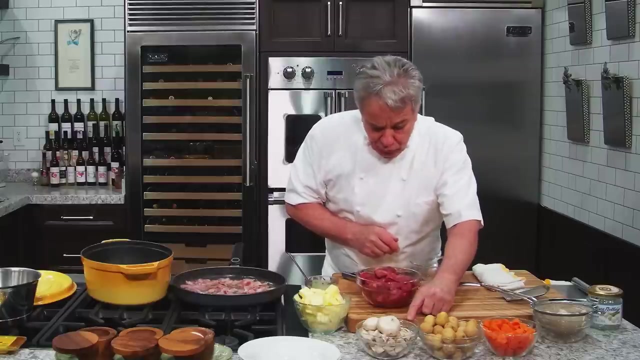 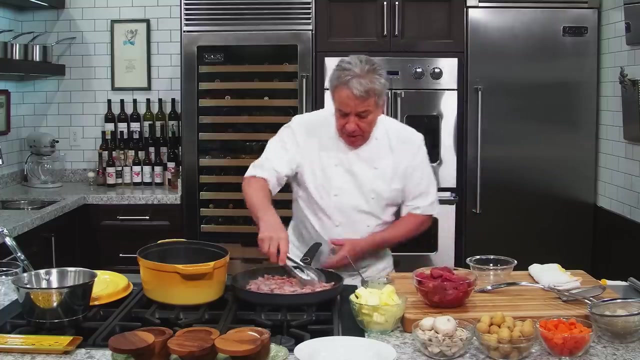 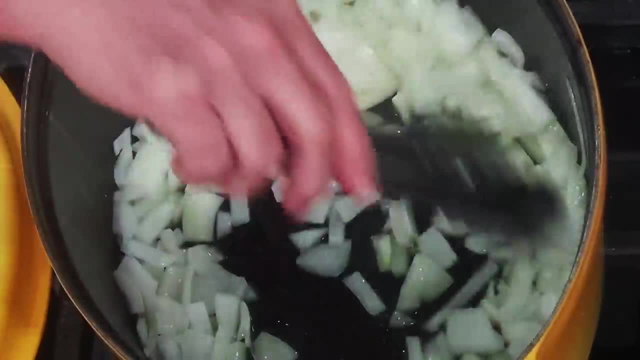 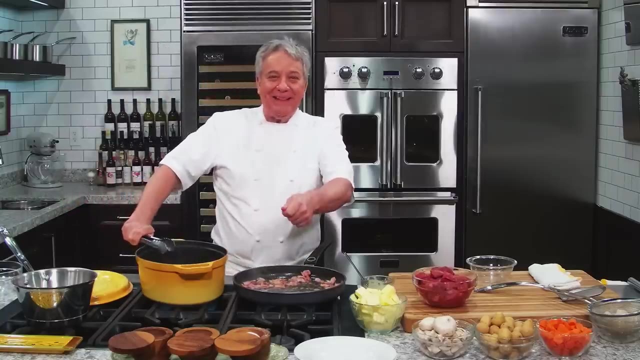 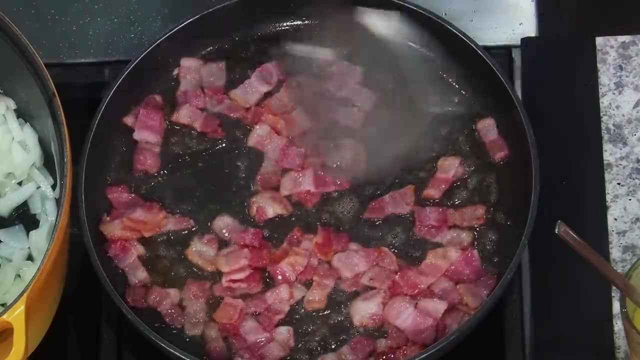 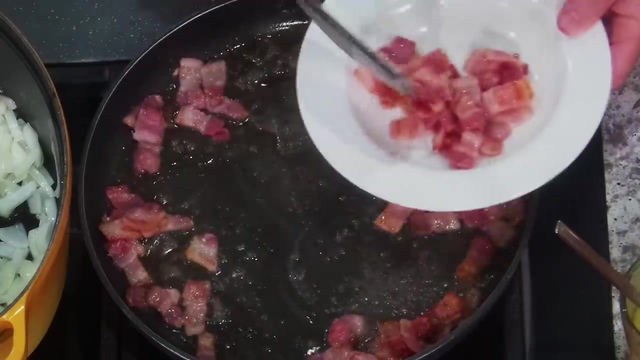 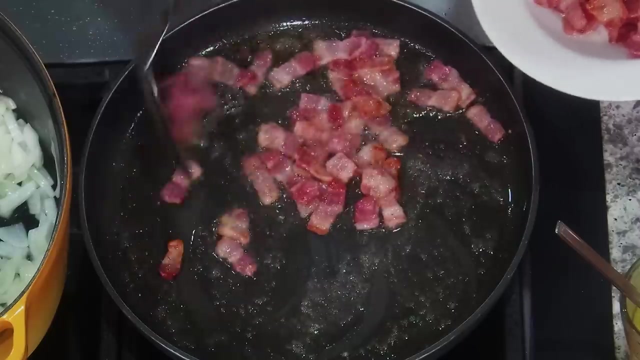 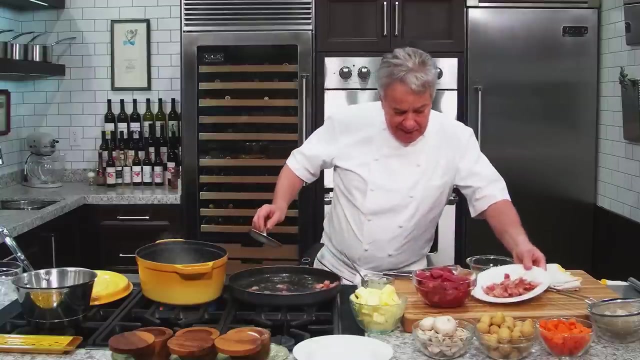 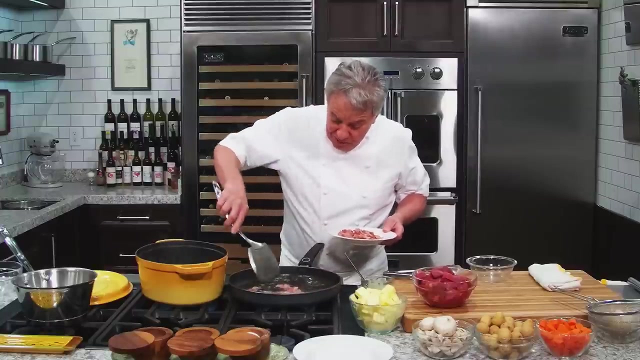 Thank you for watching and thank you for subscribing. You guys are amazing for two hours. so you don't want it to be too crispy. okay, you're not making breakfast where you want crispy bacon. let me just reduce the heat just a little bit, so the clarified butter has got a really high smoke point. the pork: 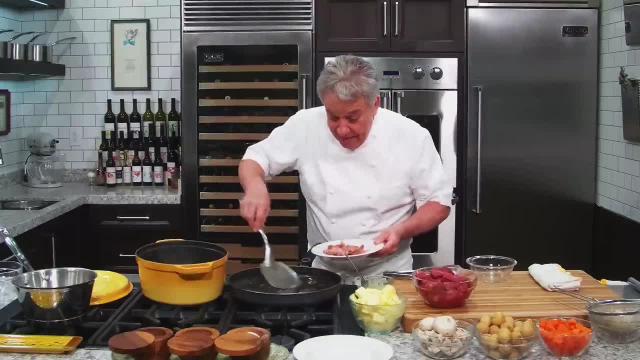 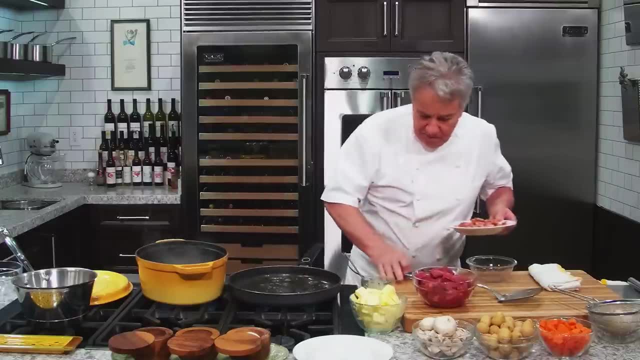 fats got a good smoke point. so you know what we're gonna do now. you know we're gonna do: friends, we're gonna saute the beef. get in here you, we're gonna saute the beef, friends. all right, we're gonna get it and we're gonna get that, Maillard. 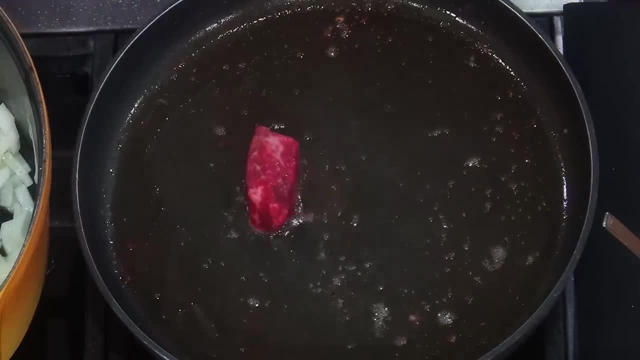 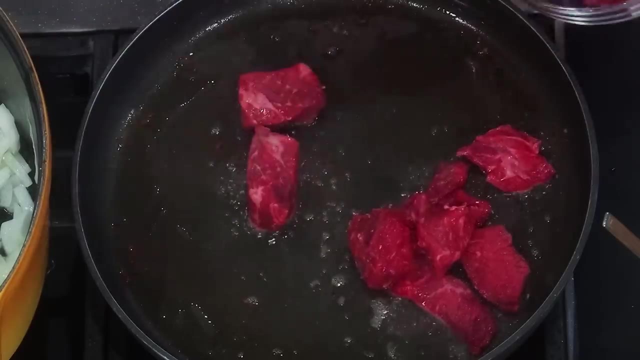 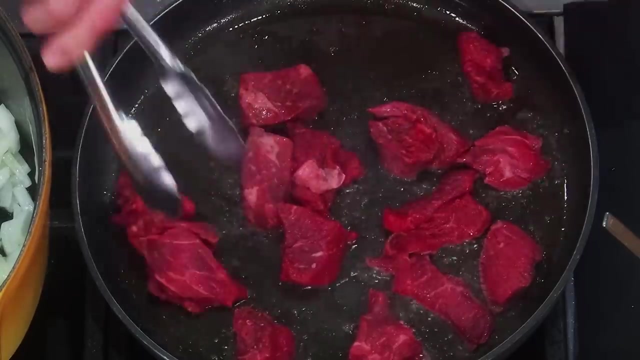 reaction. let's make sure this is nice and hot and we're gonna put the beef in here now. what you don't want to do, friends, you don't want to overcrowd it, you don't want them to touch each other. no touching, okay, no touching, we removed. 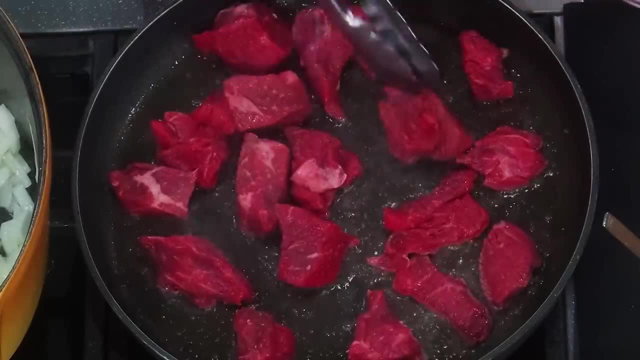 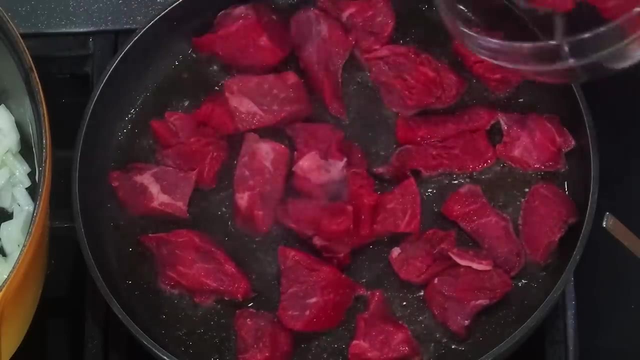 all the fat. you don't need the fat. try and make sure they don't touch each other. some- this is a little smaller. I guess when you clean the chuck roast you got to remove all the senior. what do you think I can do it? I can do it all in one pot. we want to get them too close, right? 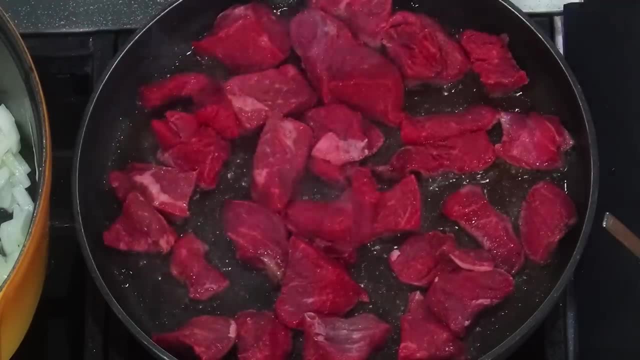 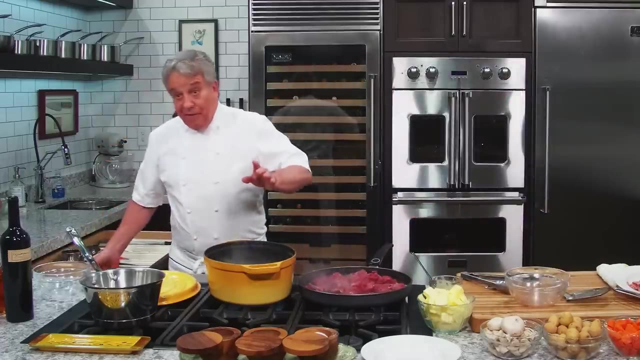 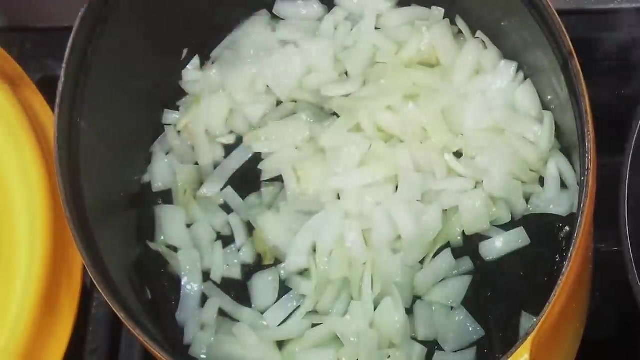 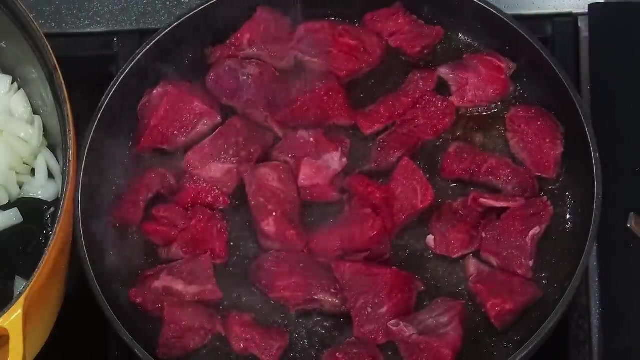 no touching if you can help it right. and now we're gonna do. let me check the onion. it smells amazing here, friends, the onion far away from being ready. before we do anything, all I'm gonna do now is I'm gonna take my soul and my pepper and I'm gonna 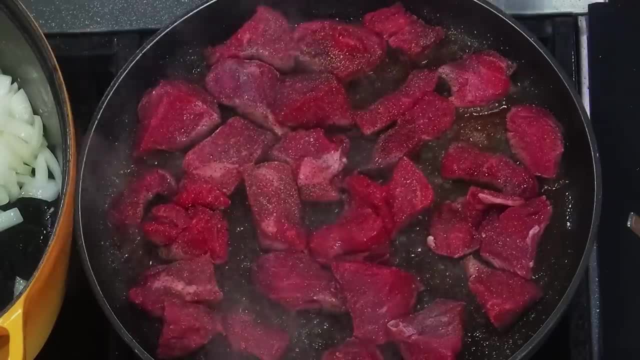 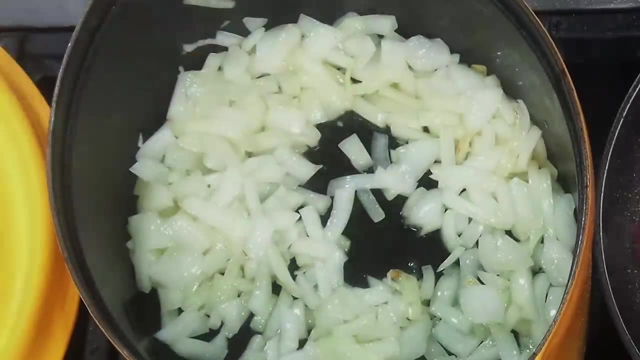 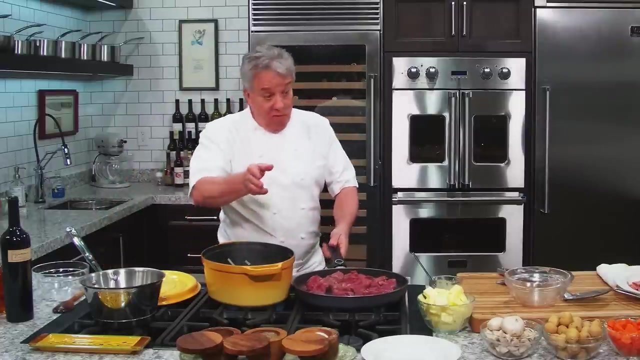 caramelize this meat. let's check it. the the onion, make sure the okay. oh yeah, you see your note. alright, you gotta saute the onion first. I keep repeating it and repeating, and repeating and I'll repeat it forever until everybody gets it in. the reason why more we said now remember when we毛煮肉. 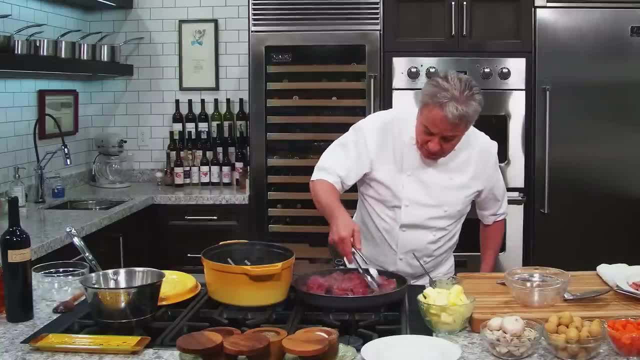 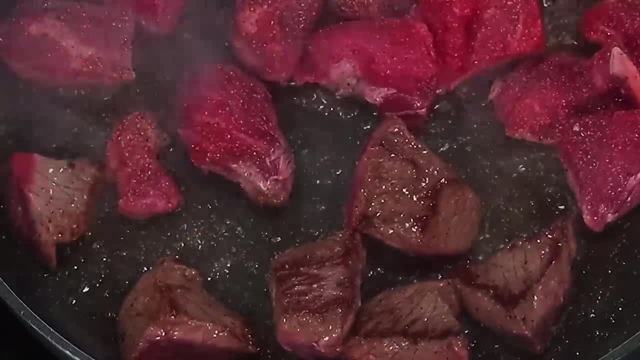 but we got a lot of people that are new to our channel friends. They've never been here before, So I don't want them to think we are too crazy. A little bit is okay. yeah, All right, look, look, look, look. 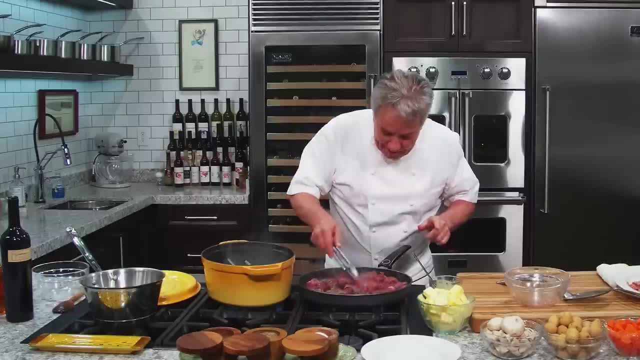 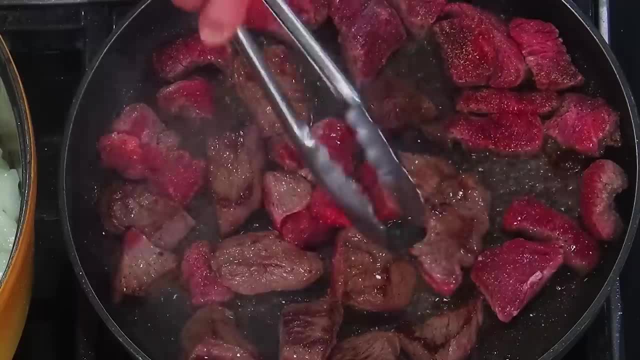 And you see, and you know what we're going to do Now. imagine: as good as that smells, right? You know what we're going to do now, friends. We're going to deglaze that pan with the wine. Oh yeah, baby. 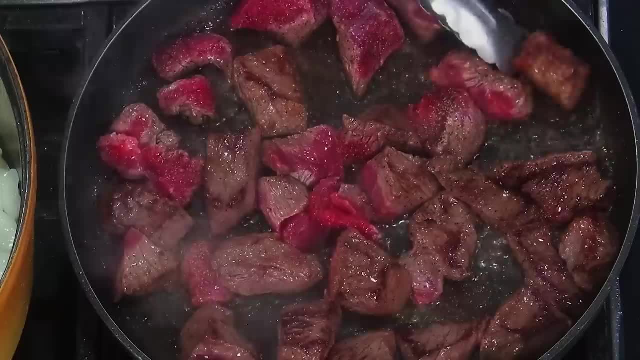 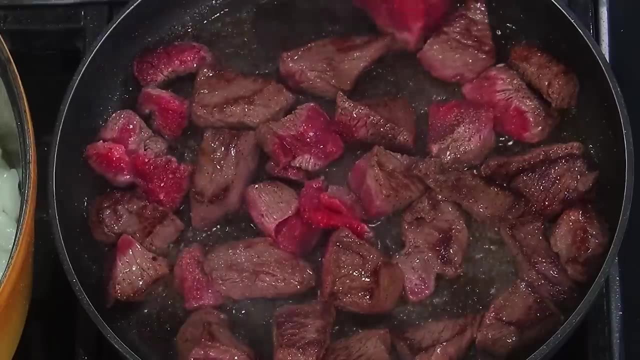 It's going to be delicious. We're going to deglaze the pan. You see that color right there. This is what I'm talking about, right there, friends. Oh man, this is hot. What a pleasure it is to cook with gas. 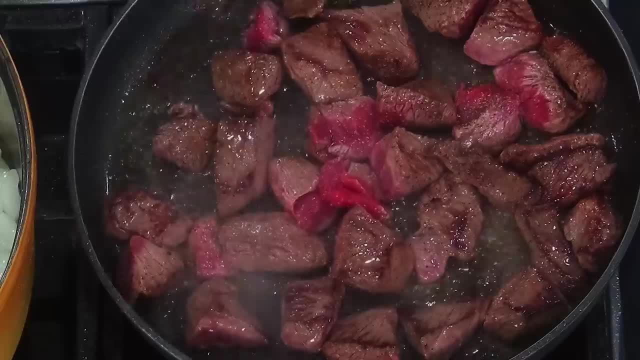 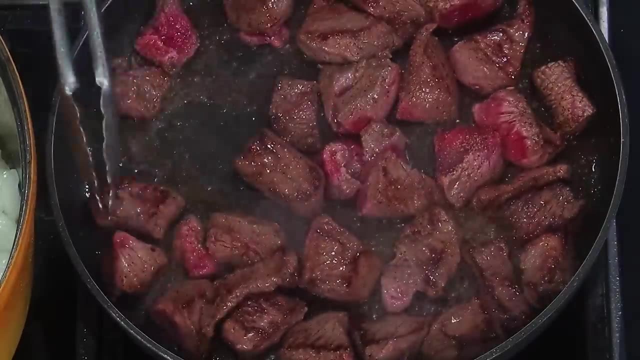 I did it my whole life. That gas, that electric stove was nice. I mean I don't want to take it down too much. It works. It helps us at the beginning. We're looking good. How's my onion doing? 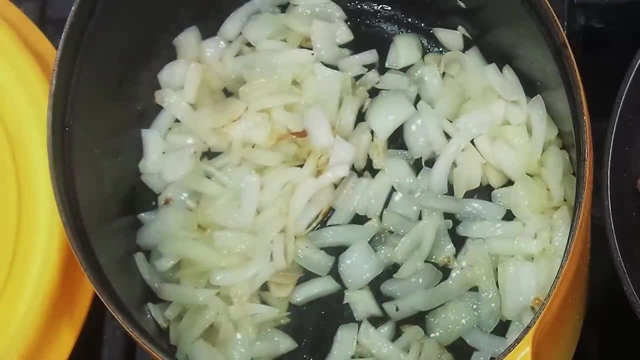 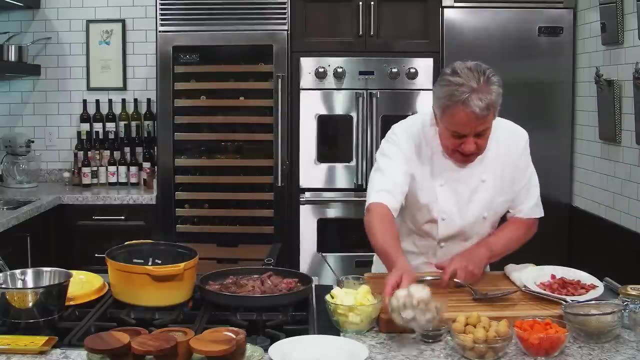 We're doing good, because you know what's going to happen. We're going to eat. We're going to eat, We're going to the next thing. The next thing we're going to do is we're going to get the mushroom. my friends, 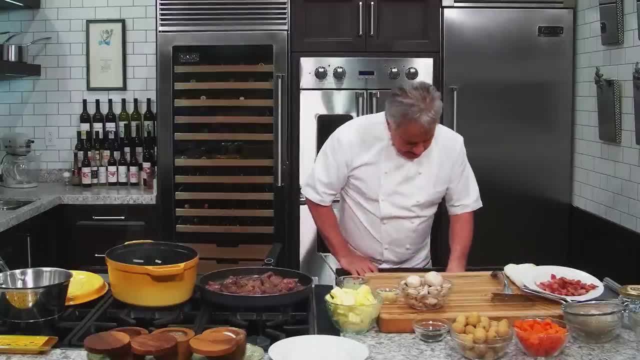 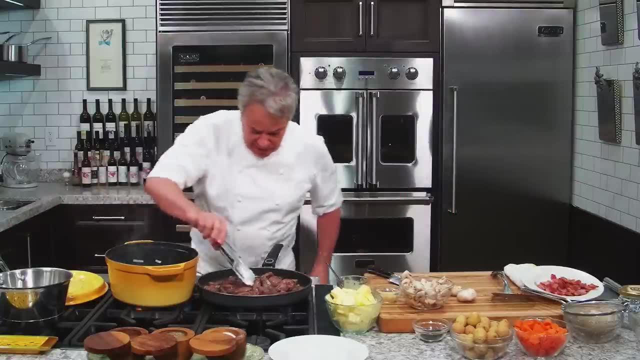 Let me get all my ingredients. I'm good, yes, And the mushrooms I just wanted to show you I like when I submerge them, which is what I'm doing here, You see. Okay, the beef is good friends. 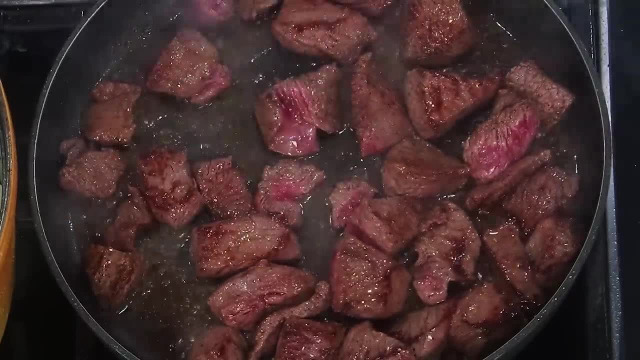 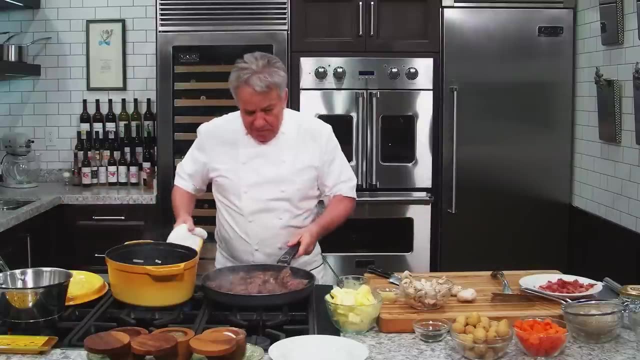 I don't want to have to worry about the beef too much. So you know what I'm going to do. I'm going to remove it And I'm going to move it on the other pot, on the other side. I'm going to put it right here because it's good. 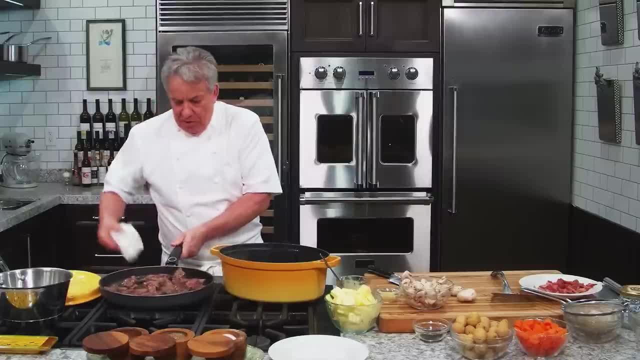 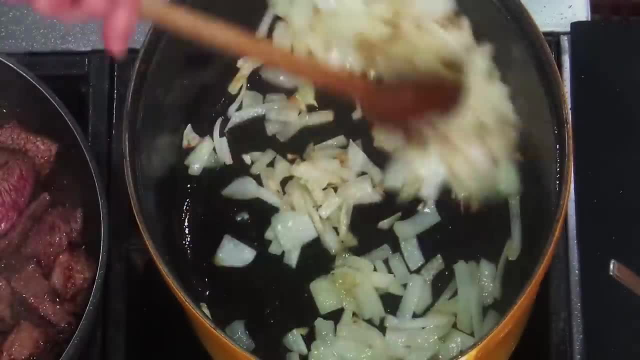 And now we're going to go here, We're going to turn the beef off, And now we're only going to concentrate in one pot. Okay, Like I said, at home I use the same pot. I just keep removing things. Oh, look, look, look. 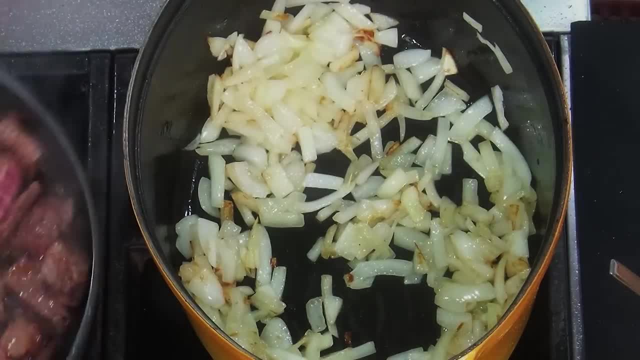 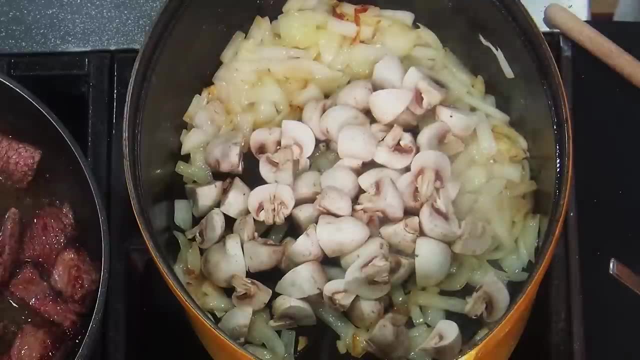 The onion are nice. See, The onion are looking really, really good. my friends, We've got to put the mushrooms in. We've got to get rid of the water in the mushrooms, So let me put them in. I want to show you. 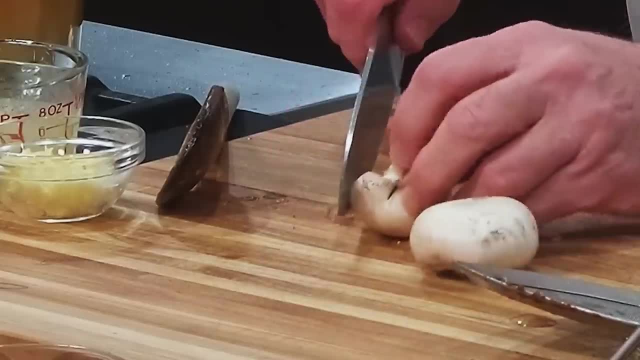 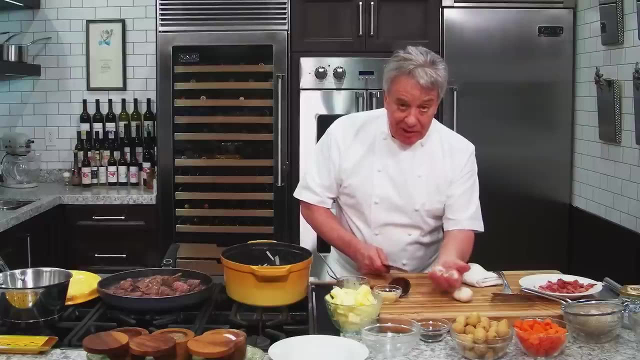 When they're big like this, you want to quarter them. Cut them in half. Cut them in half again. See, We want quarters when they're big. When they're small, you can just cut them in half, and that'll be enough. 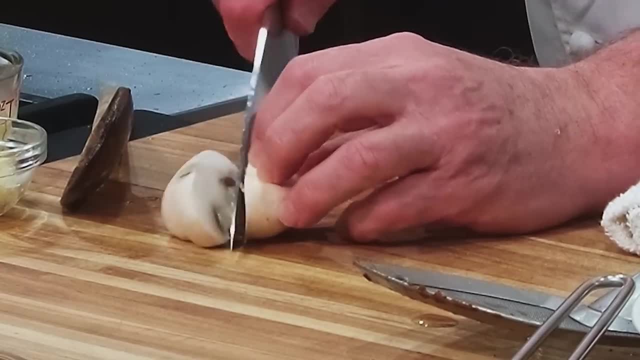 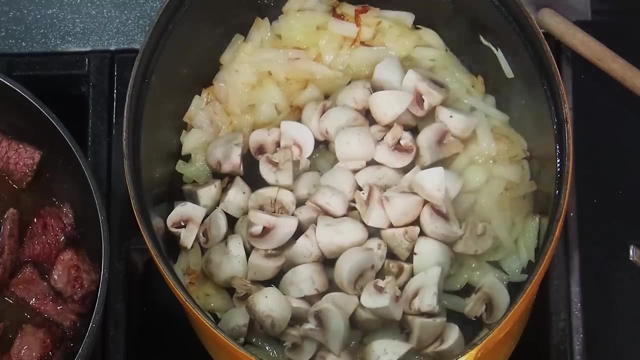 Don't miss them. When they're big, big, big like this one, you want to cut them in six pieces, And if they're too big, you cut them in eight pieces. You see, We're going to take them, We're going to put them in. 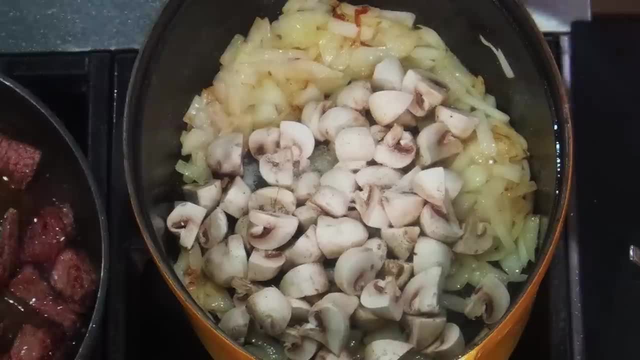 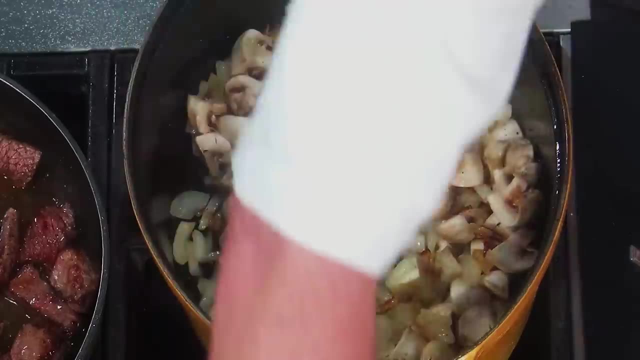 We're going to put a little more salt And we're going to saute them Until we get rid of all the water. Remember water, a little more salt, just a little bit, And that's okay because my stock- I'm going to put some stock in it later on. 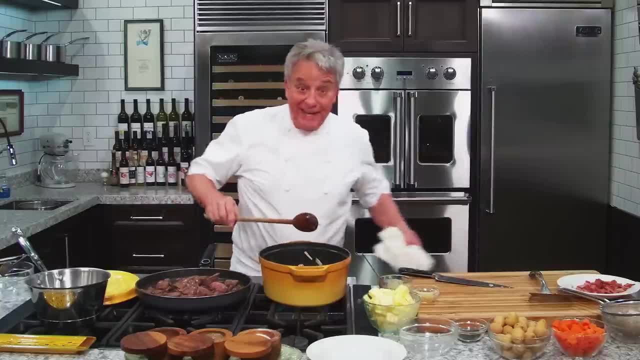 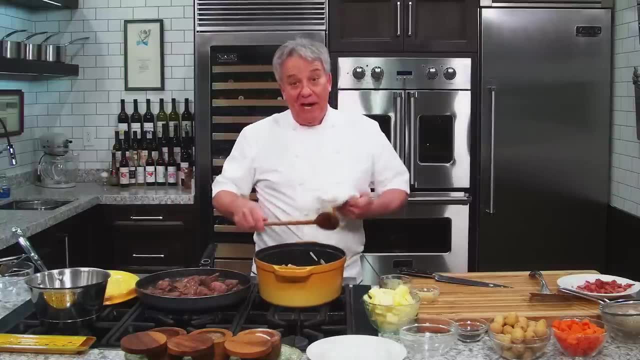 And my stock has no salt in it. Remember when you make stock. by the way, I hope some of you have tried to make the beef stock the way I showed you how to make it from store-bought, to make it a little more tasty. 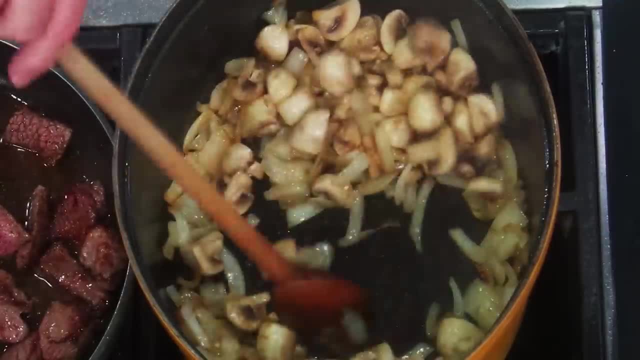 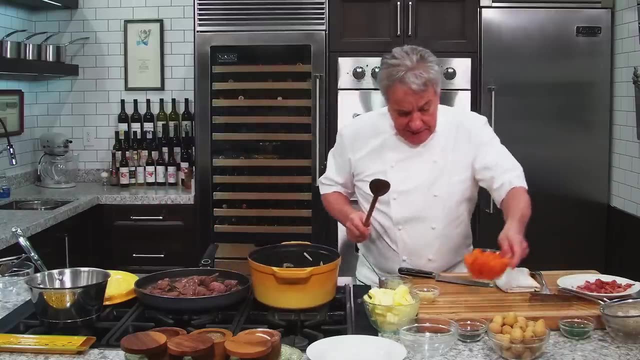 You could also add mushroom salts if you wanted to, Because we have a mushroom salt that is quite delicious flavoring. We get rid of some of the water in there And then we're going to put the carrots. Now, the little potatoes, friends, they're going to cook. 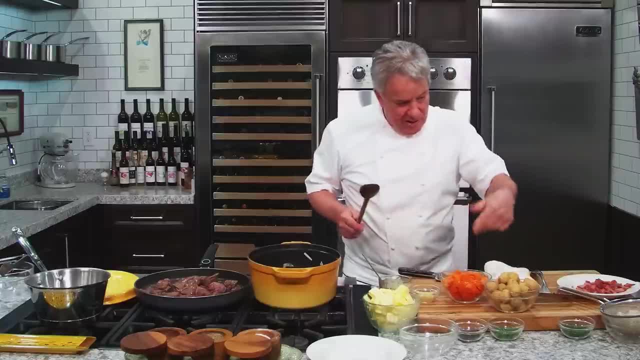 They're raw. They're going to cook at the same time, you see, And then we're going to add everything else in here. It's going to be really delicious Carrots right there. Look, everything is looking pretty good, my friends. 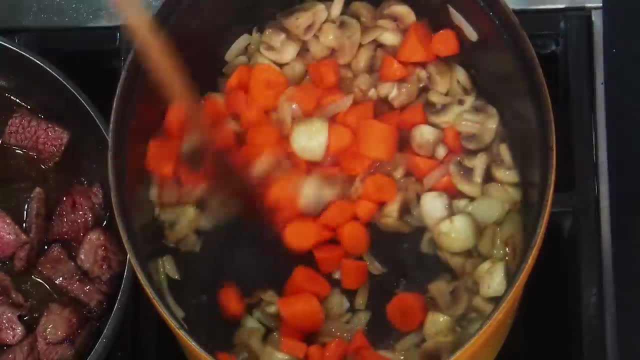 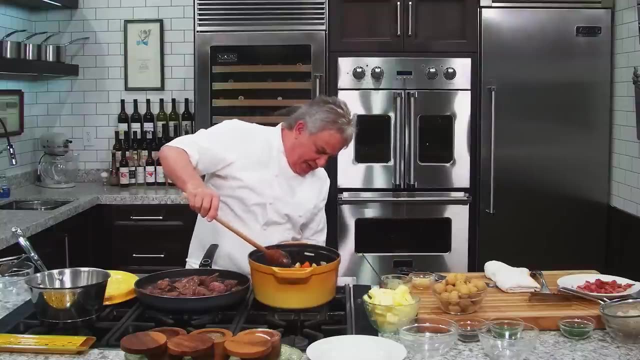 See right down there, Put the carrots in there, Saute. We're looking really good. Carrots don't need to, They should be sauteed. I just want to get rid of as much of the water as possible from the mushroom. 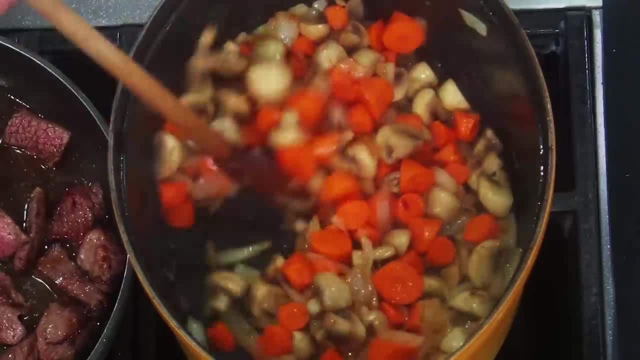 And you see, right there it's doing it. If we don't get rid of the water now, they're going to have a terrible texture. We might as well put canned mushroom. Oh no, you don't want to do that. 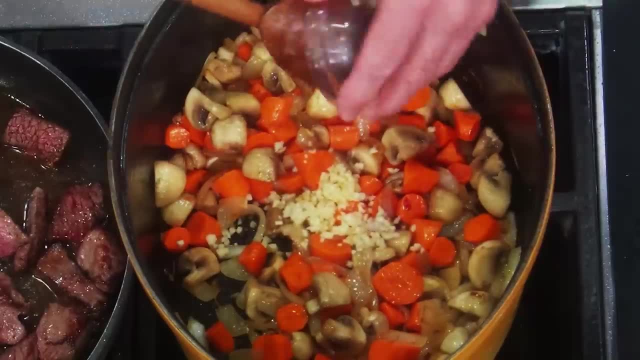 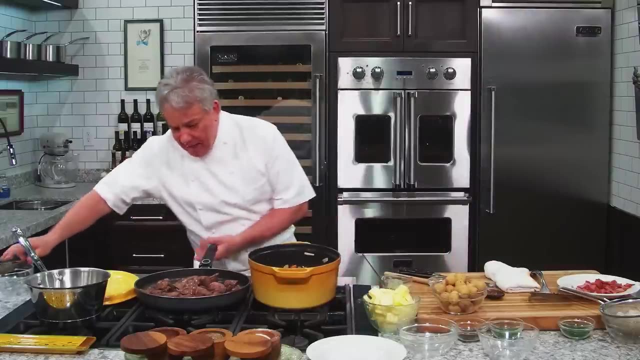 No, no, no, Don't want to do that, All right. So a little garlic in here, That's a good sign. if we put garlic, That means we're getting ready. friends. When we put the garlic, that means we're getting ready to put liquid. 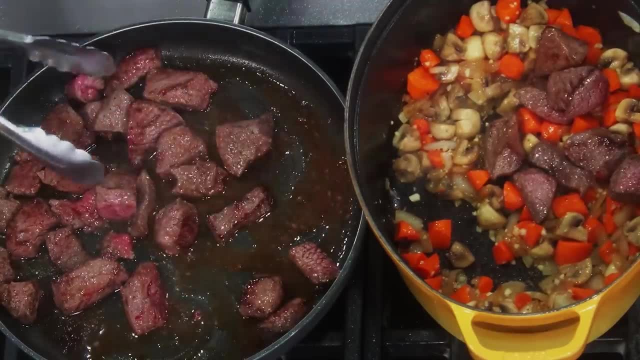 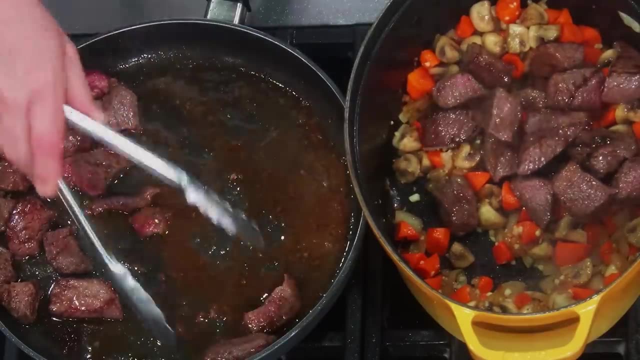 Oh, don't worry about that liquid right there, friends, I'm going to use it all, That liquid down there. I'm going to use it all. I'm going to deglaze it with the wine. Hey, look at that. 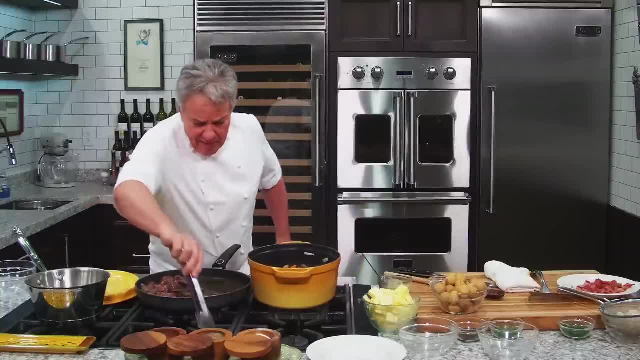 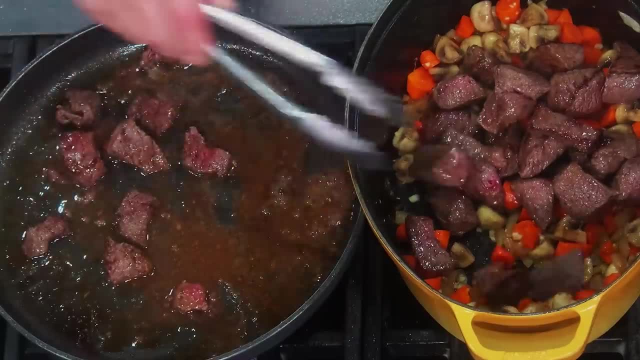 I see a mushroom down there. Oh Oh, It won't come Here, it goes, Get in here. Oh yeah, right there, baby, This is going to be good stuff. right there, my friends, I'm telling you. 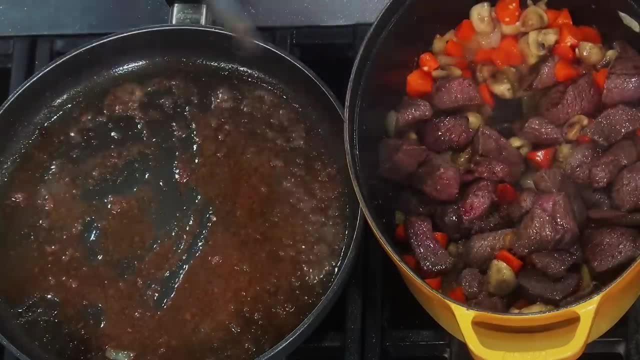 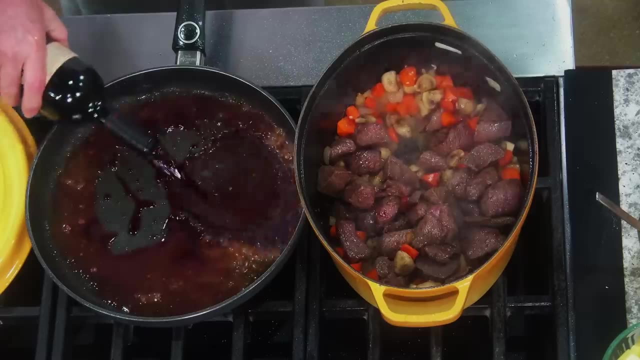 This is all goody. right there, I tell you it's a piece of beef. yeah, All right. So here we go Now. we're going to take this right there, this beautiful juice right there, and we're going to put some wine. 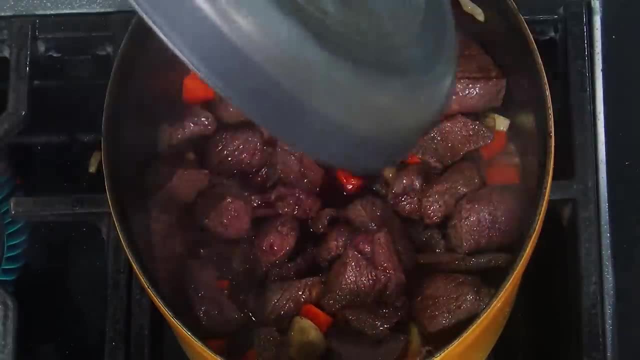 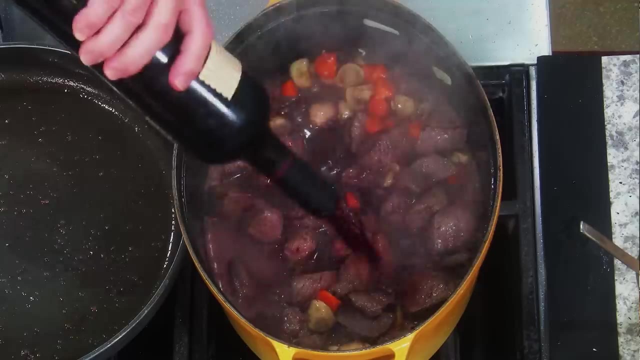 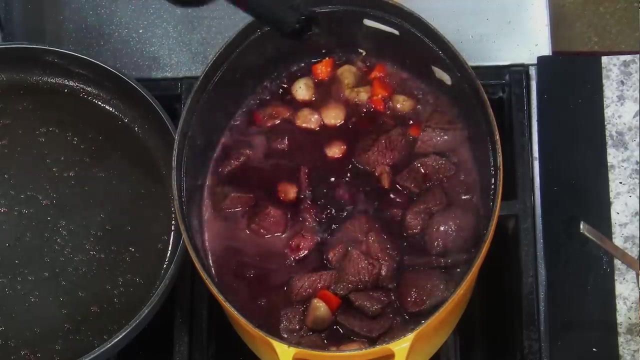 Now, beef bourguignon is definitely friends. yeah, don't be afraid to put wine. okay, I serve a glass for me. Oh, I guess I'll open up another bottle, A whole bottle of wine, And then we're going to put some cognac at the end. 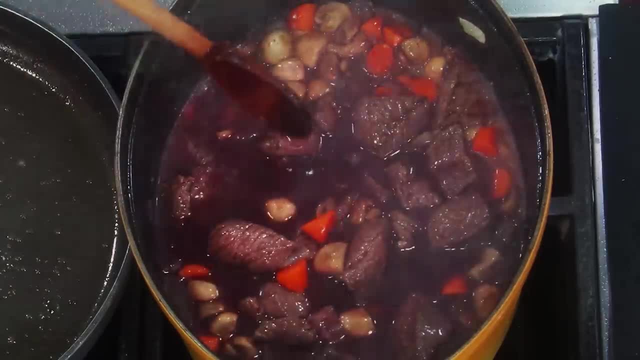 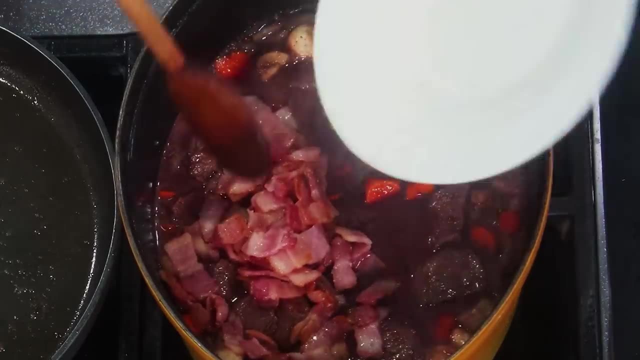 Oh yeah. So the only thing that we haven't done yet, we have not sautéed the pearl onion, the bacon, Get in there. Oh yeah, baby, Yeah, this is going to be delicious. Like I say, you don't eat bacon, don't worry. 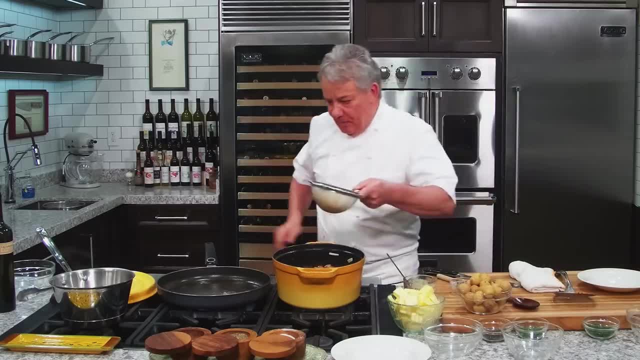 You don't need to put it in. You just don't eat it anyway, right, So you don't need to put it in. Make sure your pan is hot. We're going to sauté those caramelized onion just to give it a nice color. 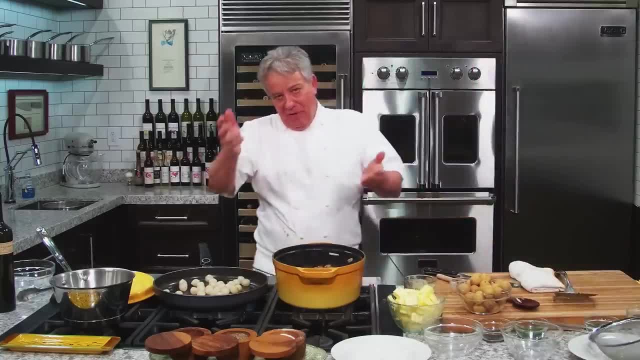 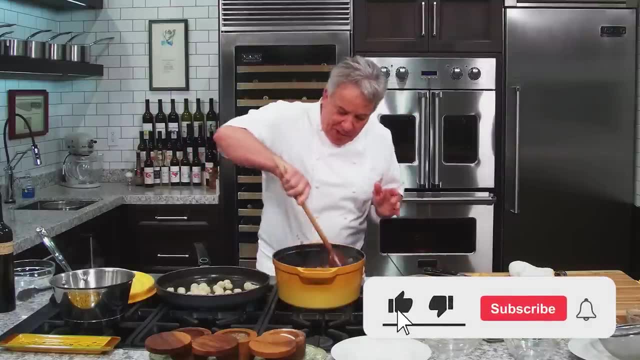 You can skip the caramelized onion. You're already Got some onion on there, if you don't want to. Now, my friends, here's two things we're going to do. First, before I'm going to put a little broth in here, 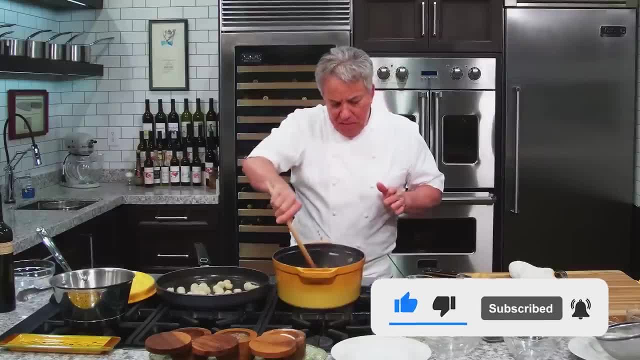 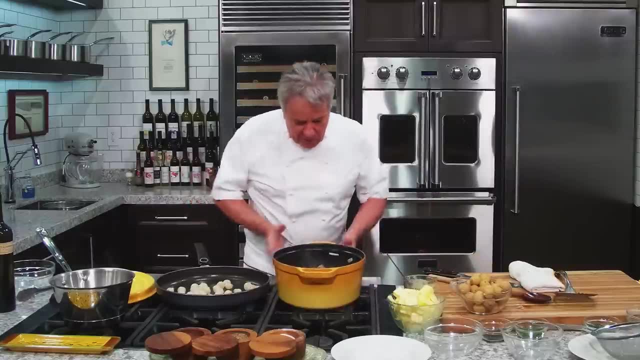 But before I do that, I want to reduce my wine and try to get most of the alcohol out. That's much better. So we're going to do a wine reduction. We're going to bring the whole dish to boil, right. 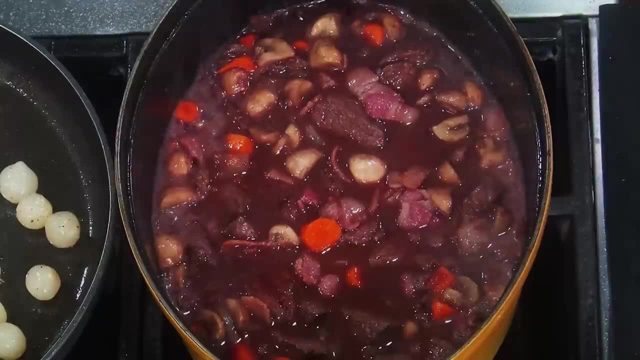 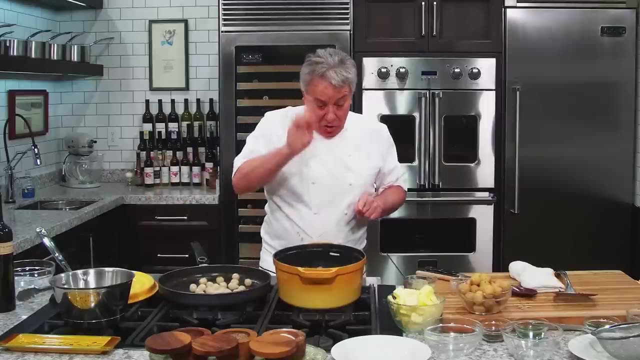 We're going to bring it to boil, We're going to let it come to boil, We're going to reduce the wine, And while we reduce the wine after that, we're going to put a little bit of stock. So, not to make the video too long, we're going to stop filming right now. 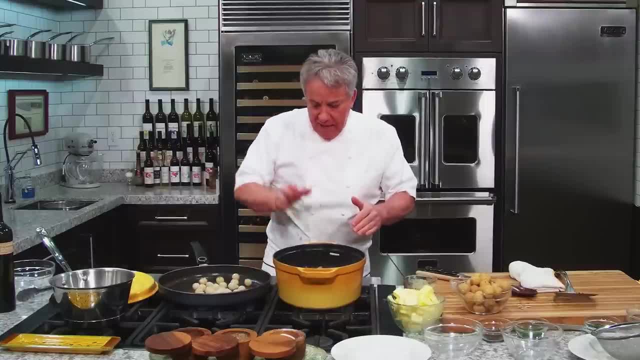 We're going to let the wine reduce And I come back in about two or three minutes. The caramelized- the onion would have caramelized. We'll add them to this, We'll add a bit of stock And then I'll show you how to thicken it. 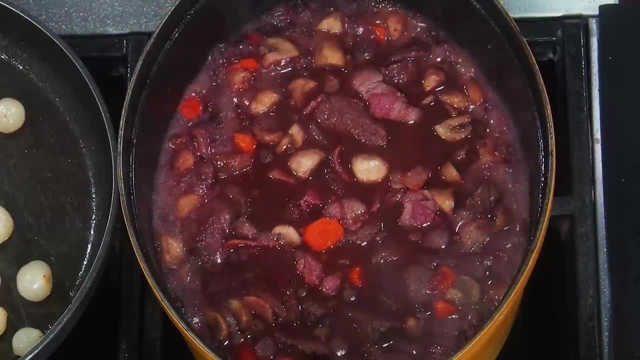 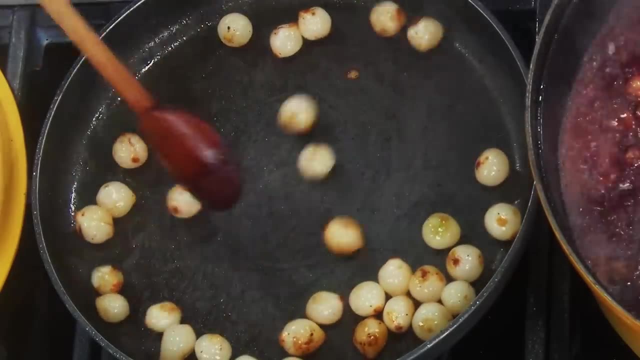 So we'll be back in about three or four minutes, however long it's going to take to reduce this wine. Okay, All right, friends, Look, look, Look. how beautiful the caramelized The onion. see, the onion has caramelized. 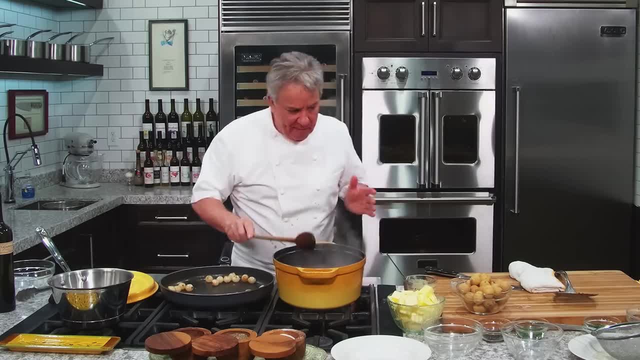 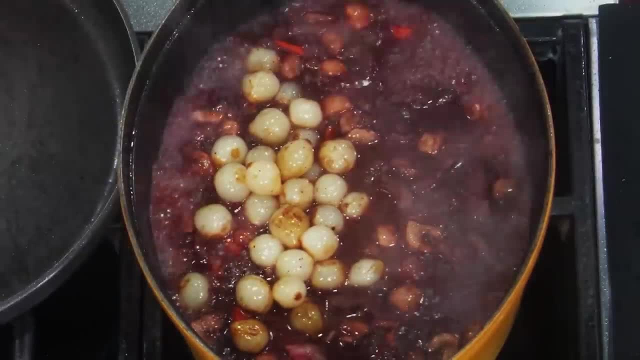 It's got a nice flavor. We can turn them off. The wine has reduced enough. Okay, just two or three minutes. You want to get a nice reduction, right? We're going to put the onion right in there, And I didn't leave myself any wine. 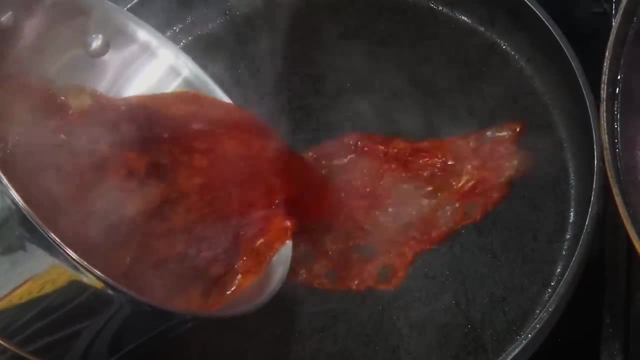 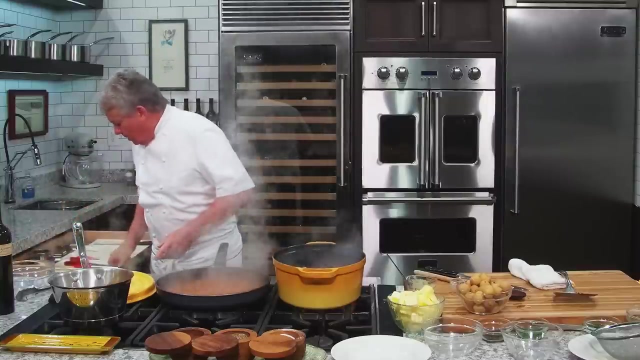 So you know what I'm going to do. I'm going to deglaze that pan with a little bit of broth. This is my beef stock. This is the beef stock that I was telling you about. Let me clean up the pan really good. 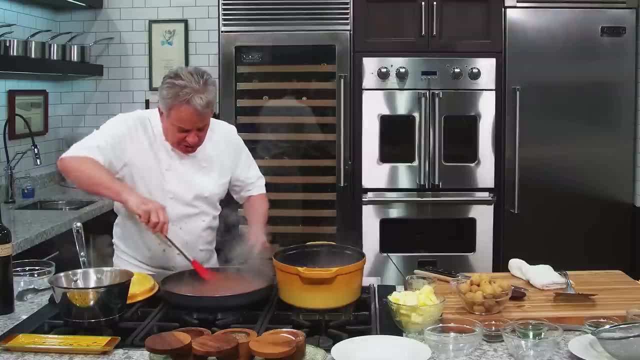 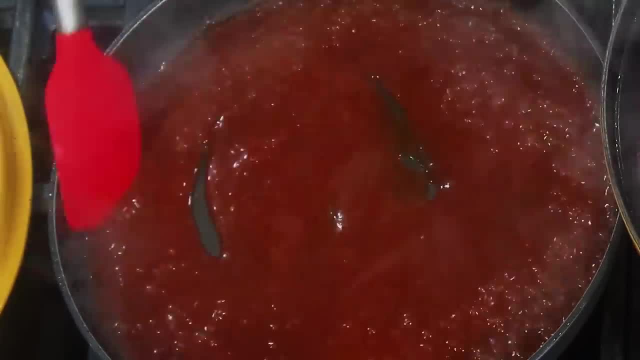 The heat is off, It's just the remaining heat. Just to clean the pan. you see, It's just to really, really clean the pan. Antonio's going to be very happy because I cleaned the pan. See: Clean the pan. 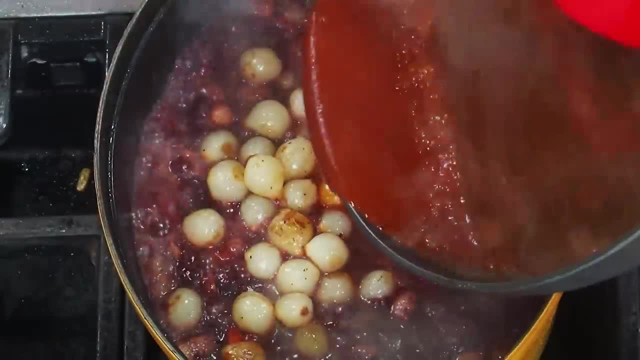 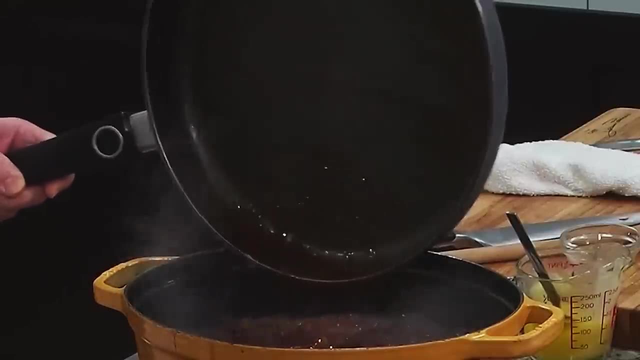 See, look, look. And now all these goodies, friends, You know how good that's going to make it. Yeah, That's going to be so delicious. my friend, Look at this, That fry pan is brand new clean. 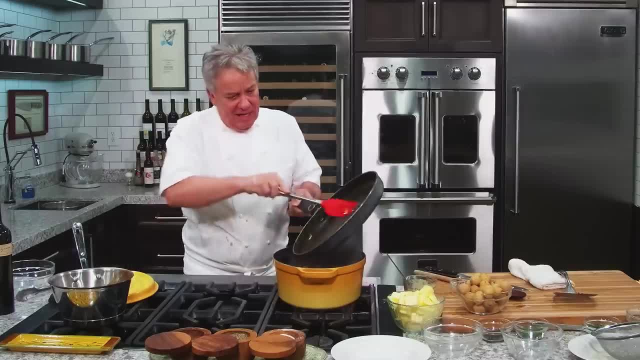 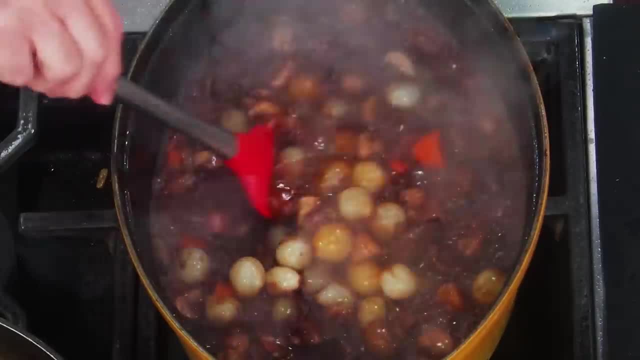 See, Look at this, Look at this fry pan friends, It's clean. You see, There's nothing, Nothing, Nothing, nothing, nothing, nothing, Nothing left in there. So now let's reduce the heat. Let's reduce the heat. 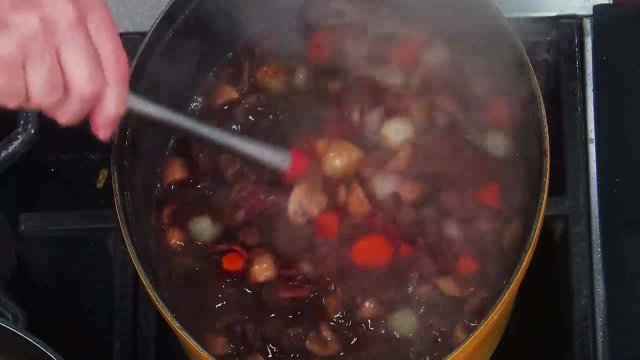 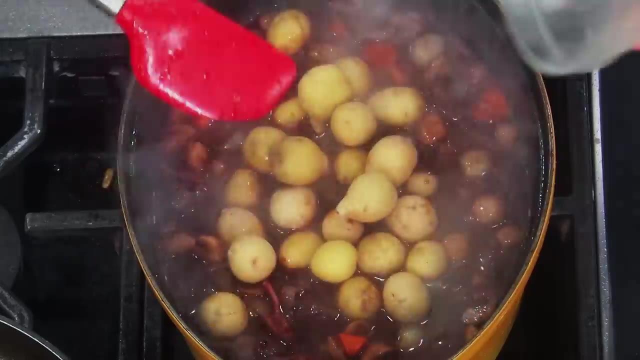 So far very simple. Why do you notice? Very simple. Now we're going to put the potatoes. You let them cook in it. Let them just cook them right in there. Those little potatoes, I got little potatoes. You don't have those little potatoes? 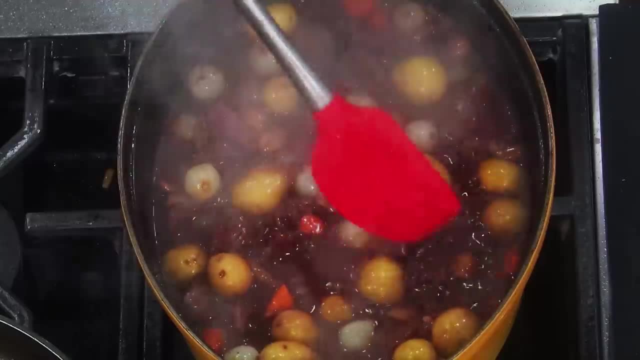 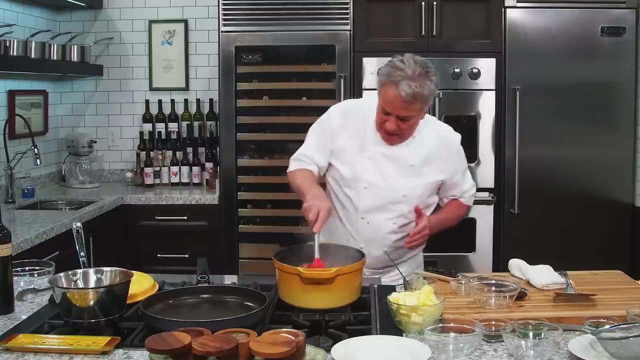 You can get whatever potatoes you can find. You can cut them. You don't have to put potatoes. You can serve with mashed potatoes. I also love it. I also love it with the mashed potatoes. Okay, And it's up to you really. 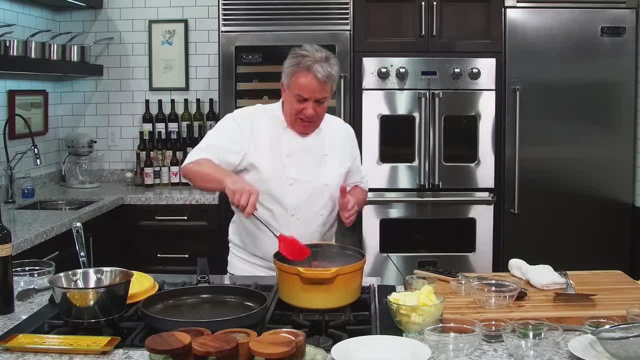 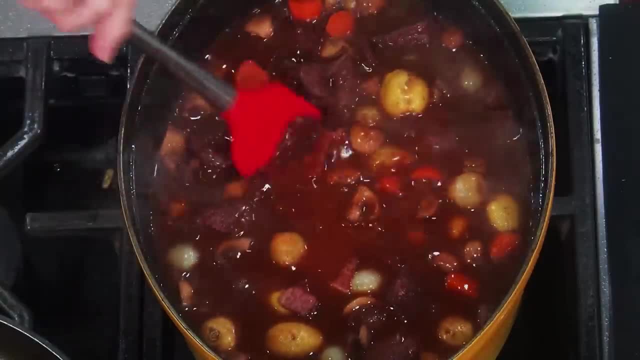 I just love to serve it with some kind of a potato. So, mashed potatoes, Let me put just a touch more stock. There you go, And this right there, my friends, is. So now let's talk about thickener. 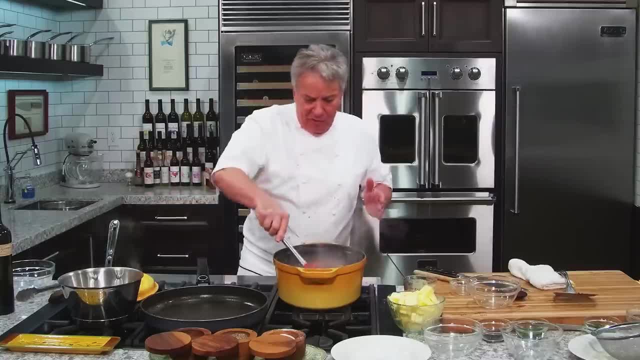 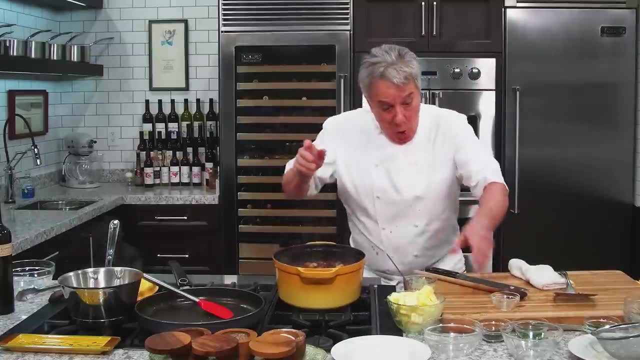 If you watch any of my other videos- the beef stew and all that- you already know how to do this. But you see a lot of people. what they use, they use a beurre manier. Oh, mamma mia, Oh, thank goodness I'm here. 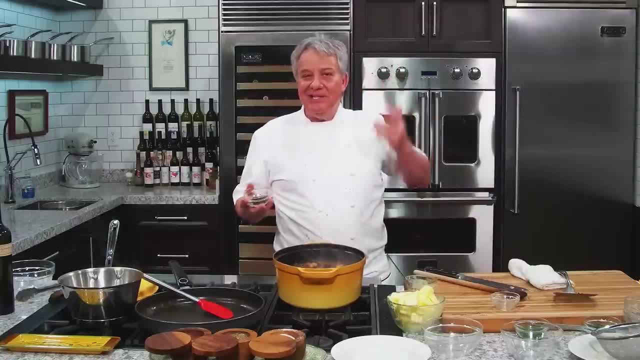 Thank goodness I'm here, And where would I be In another kitchen, somewhere Where I'm cooking for you? I forgot fresh thyme. You got to put fresh thyme, Fresh thyme. If you don't have fresh thyme, then use dried thyme. 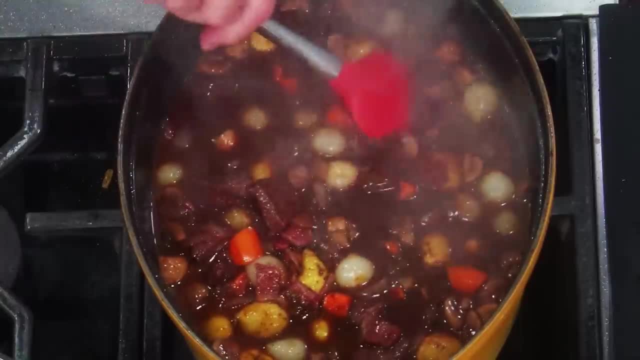 That's okay, It's really important. Okay, I put the garlic in there. right, I hope I did Ay, ay, ay. Sometimes I forget I put salt and pepper. I'm going to put a little bit more pepper. 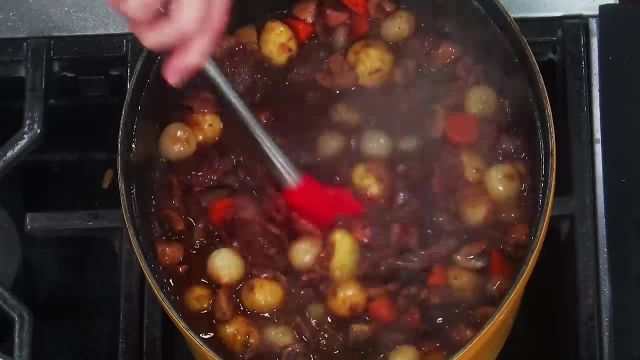 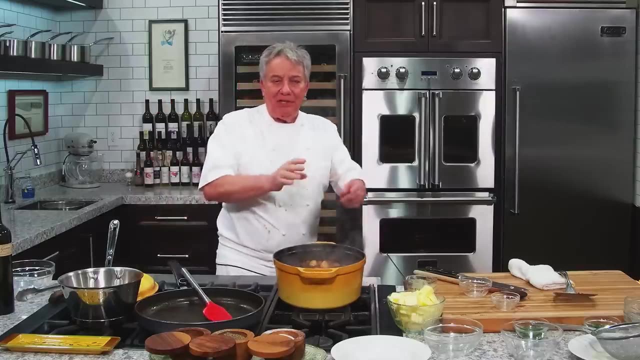 And I put a little more salt because my stock is not doesn't have any salt. Remember, It's homemade, So it doesn't have any salt. Salt, salt, salt. All right, So you can put a beurre manier, which is butter and flour. 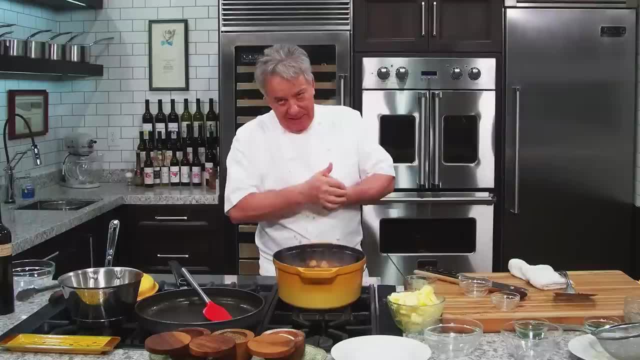 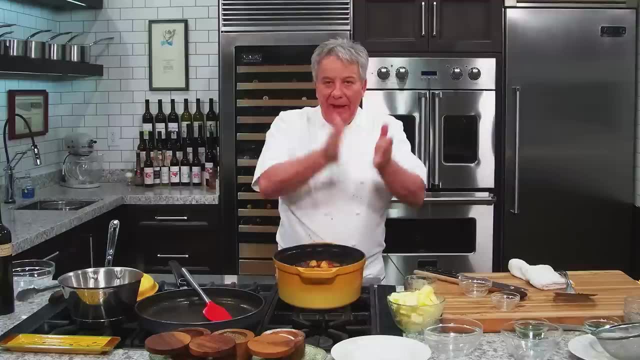 You mix them together. I don't believe in that technique. Okay, I don't believe in a technique. People, especially people, do it at the end. It's not because the butter is mixed with the flour And if you put it at the end, then it's going to the flour flavor is going to disappear. 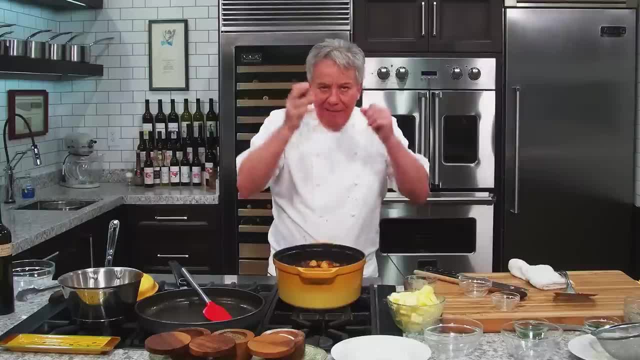 It's going to be starchy. It's going to taste like glue. Flour needs to cook. You're going to put flour. You got to put it at the beginning or you got to put it at the end, But it's got to be. 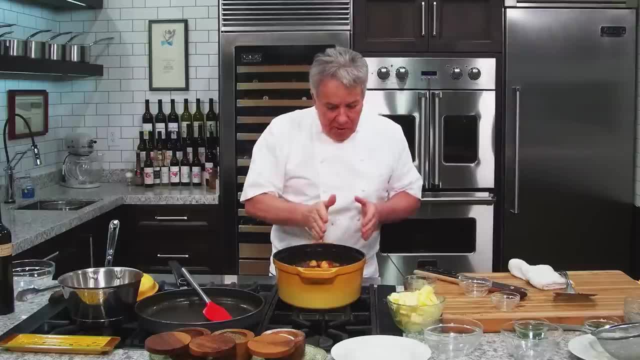 It's got to be cooked roux. We'll talk about that another time. All we got to do now we're going to put flour in there. Now, how do we do it? Dilute it in water? No, we don't do that. 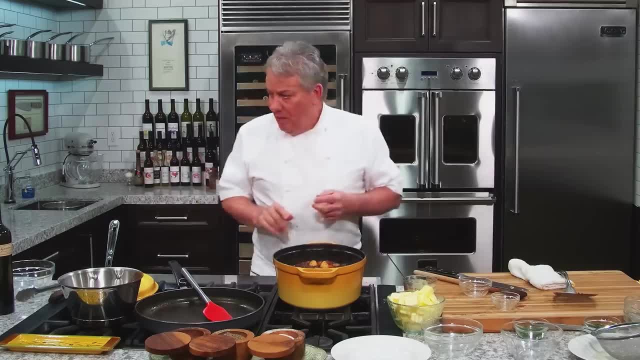 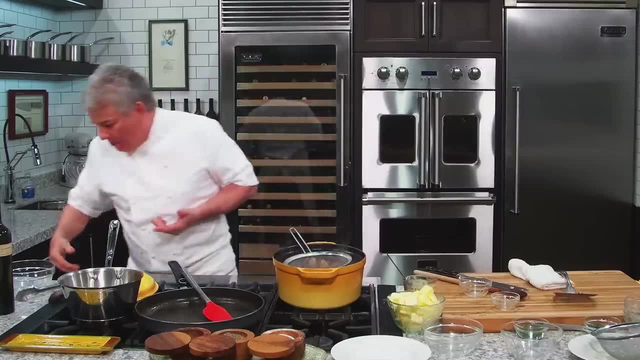 So, for those of you that have been following my channel, you know where I'm going with this. I'm going to put my strainer. And for those of you that have never seen this, this is a cool technique. I promise you you're going to love it. 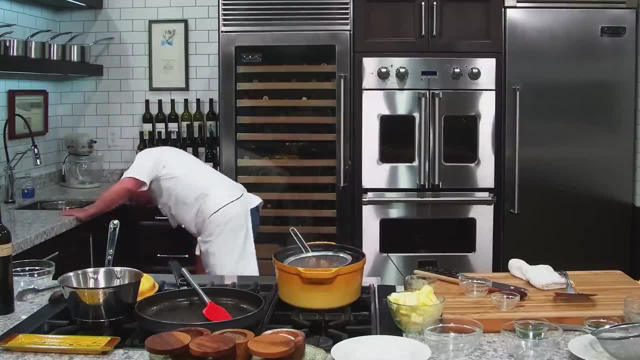 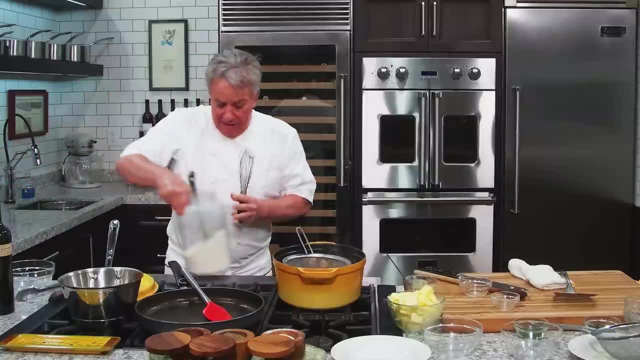 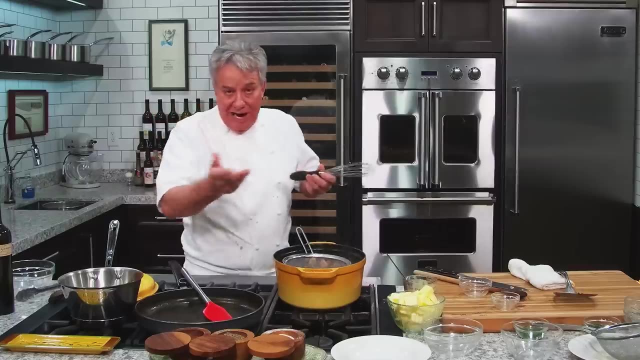 I got to get a whisk, And then I'll show you. All right, I'll show you. It's very simple. We put a strainer in there And then we'll put flour, Okay, And then what's going to happen is the flour is going to cook for the next two hours. 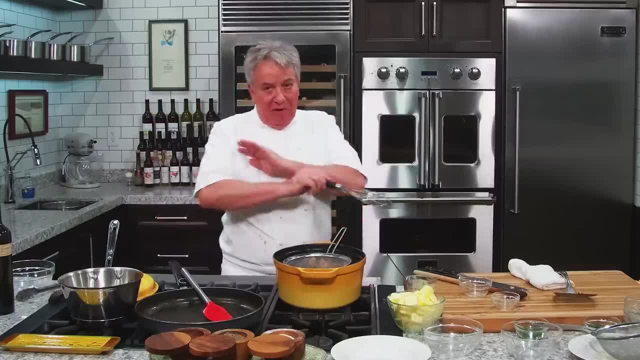 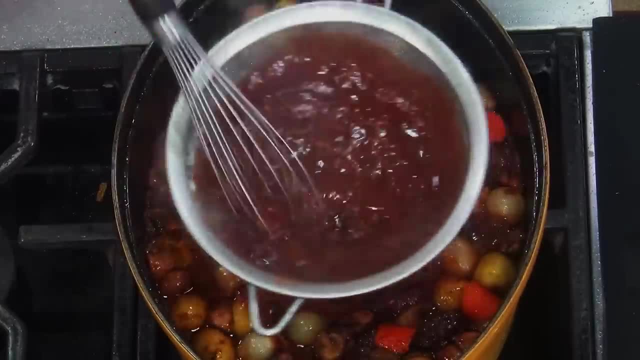 Two, two and a half hours, However long it's going to take for it, And I promise you the flour you'll completely, completely disappear. What you do, you just mix it up in here like this. You see, If you've seen the channel, you've seen me do this before. 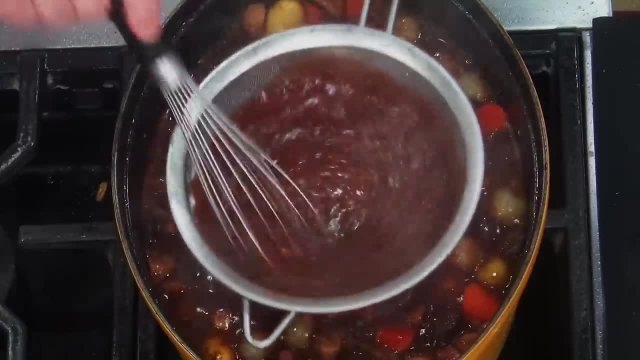 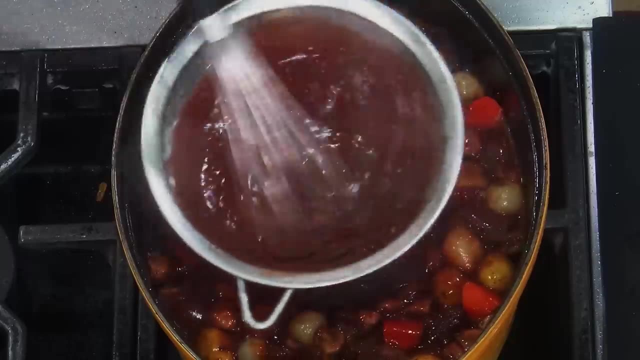 And it's a really cool technique. If you've never used it before, I highly recommend you try it. You know I've been doing this my whole life, friends, And I'll tell you what I've used- every thickening technique you can think of. 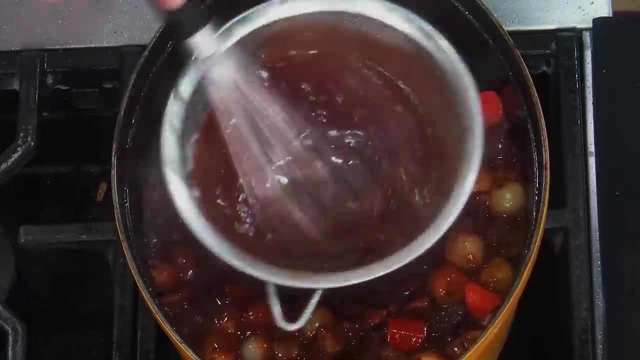 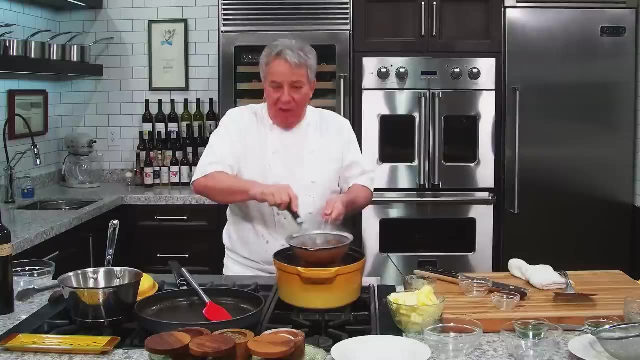 Okay, And a cornstarch, Arrowroot, Tapioca powder And beurre manié Rue, Cooked rue, Not cooked rue, And this is an easy thing for you guys to do at home, But also, if you're not new to the kitchen, if I say, oh, let's now use a rue. 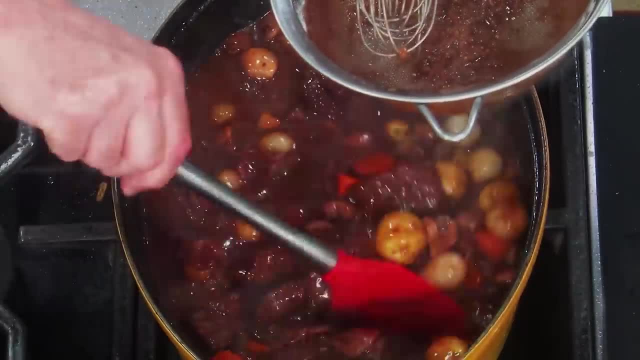 You're going to say: well, I don't make a rue. Of course you don't make a rue. Most people at home don't make a rue. We got to be realistic. This is not a channel that is about me showing what I can do. 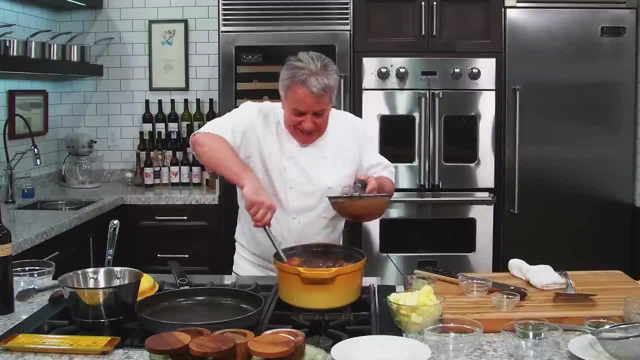 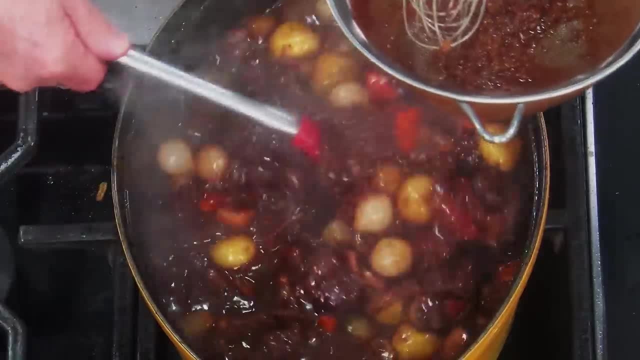 About me getting you in the kitchen to do these things and be successful at it, Because it's not that difficult to do. So let's look at it. Let's see how thick it is. See, It's a little. it's still a little liquid. 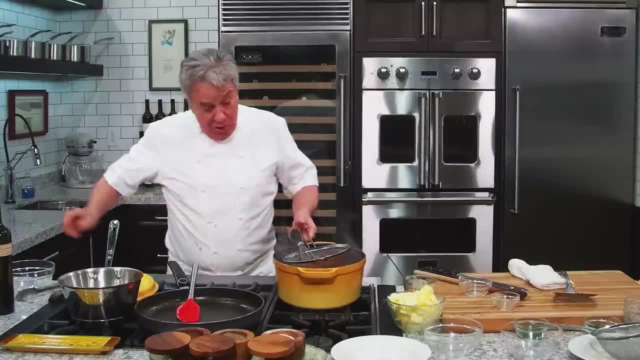 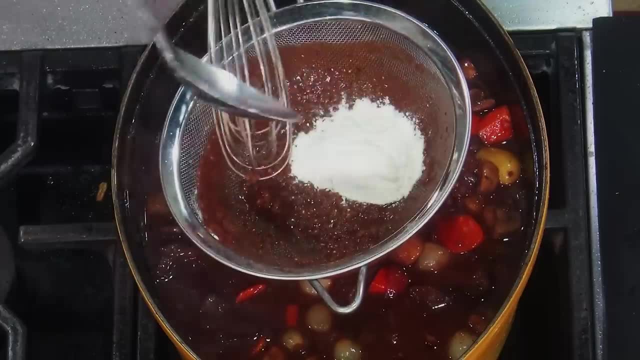 We're going to put just a little bit more. Be careful now. If you're going to add more, you can add more to all the cooking. At least you got to give the flour at least 15, 20 minutes to cook. 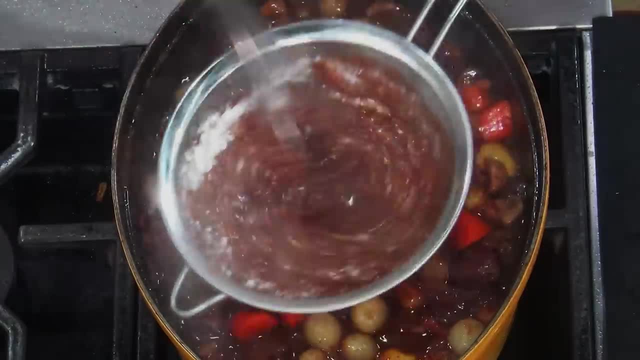 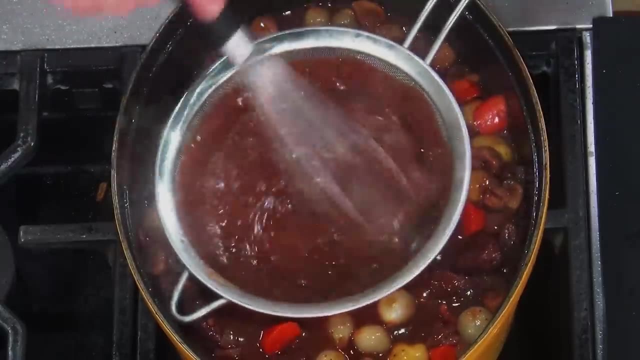 So up to 15,, 20 minutes, until you. When you're finished, you can add a little bit more flour. okay, But don't do it at the last minute, because that flour, I don't care if you add butter to it. 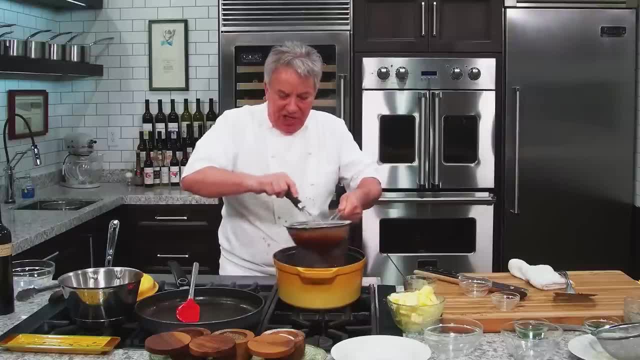 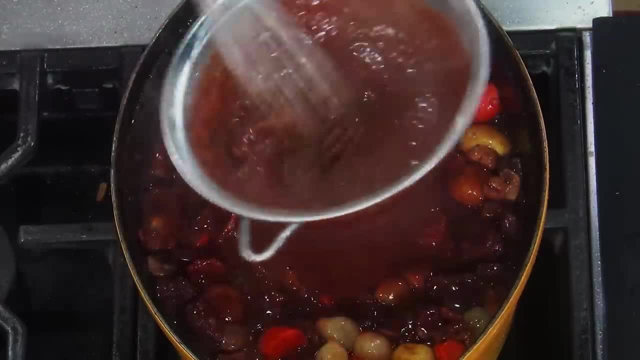 it's still not going to cook, okay, And the starchiness of the flour is not something that I enjoy, Okay. So look, Everybody can do this. Everybody can do this. This is not complicated to do, You see, And it works wonderful, my friends. 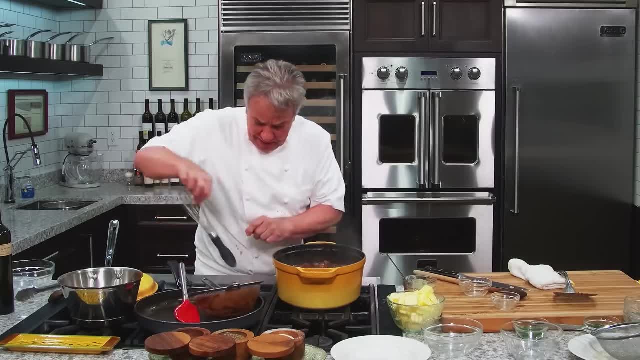 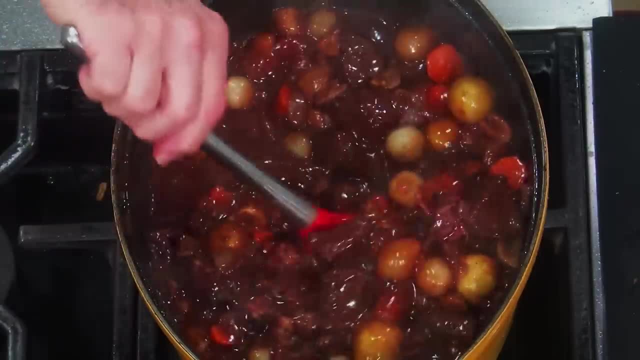 All right, Oh, mamma mia, I think we're done. You come back over here. All right, Now look. So now you can cook this in the oven, friends, You can cook it in the oven and it will cook beautiful in the oven. 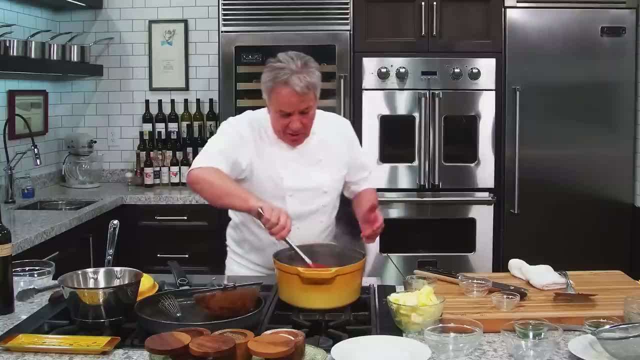 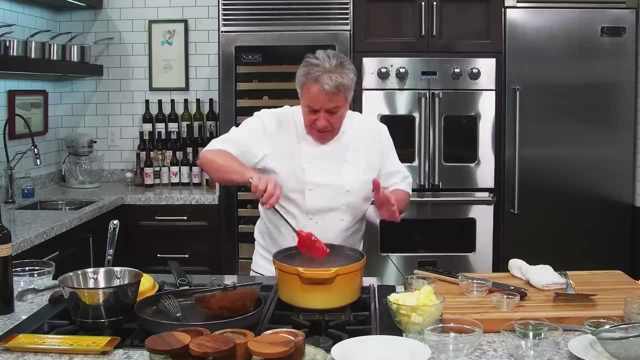 It's going to take about two and a half hours, at three and a quarter approximately. You'll check it to see when it's done. The meat has to be like fork-friendly okay, And that's all we need, my friends right there. 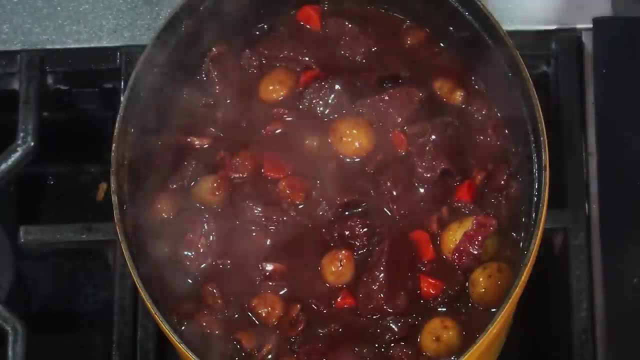 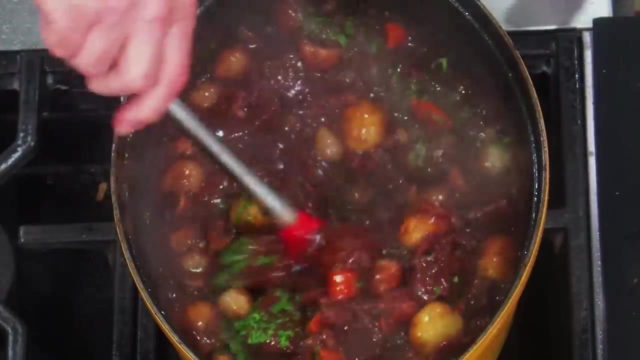 We're going to put a little bit of parsley now and then we'll put a little bit more parsley toward the end. All right, We'll get better. Now, this is each one for flavor, and the one we'll put at the end is for the look of it, because it looks nice and fresh. 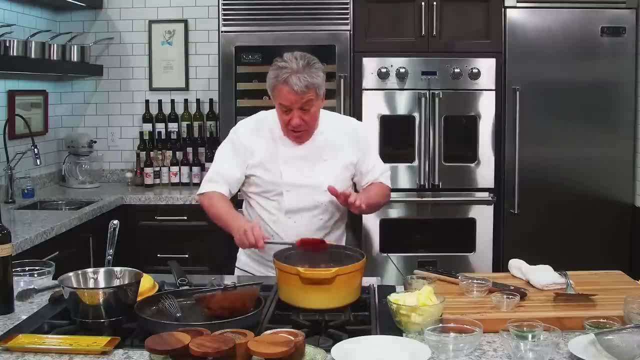 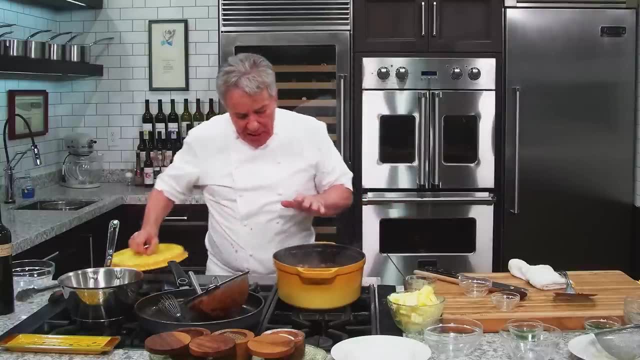 Okay. so, like I say, in the oven or on the stove. If you leave it on the stove, let me tell you it smells amazing. If you put it on the stove, you can cover it, because you're going to cook it very slowly. 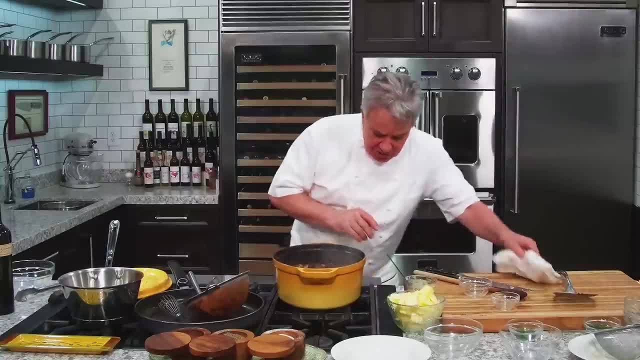 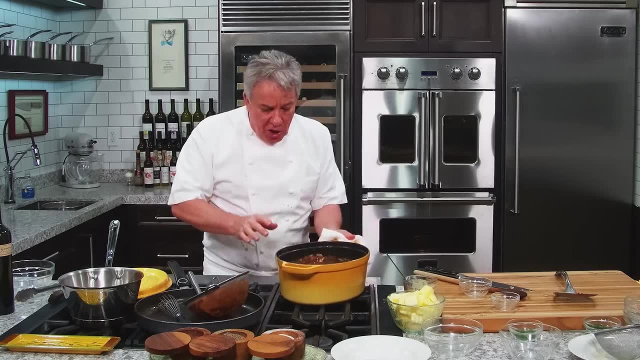 Remember this is like very low heat. Look, I'll show you the heat. I got it on. You see, Very low heat, As low as you can get. If your butter is too big, then put in another butter You want it to cook. blue, blue, blue, blue, blue, blue. 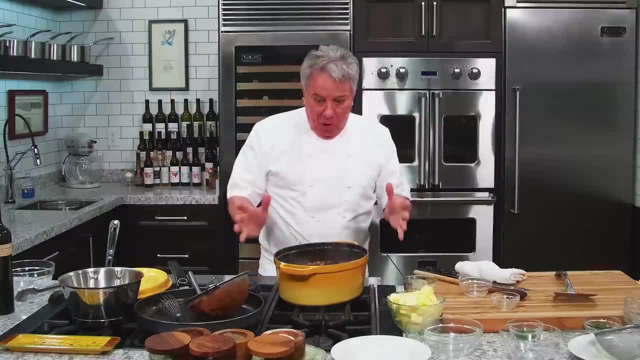 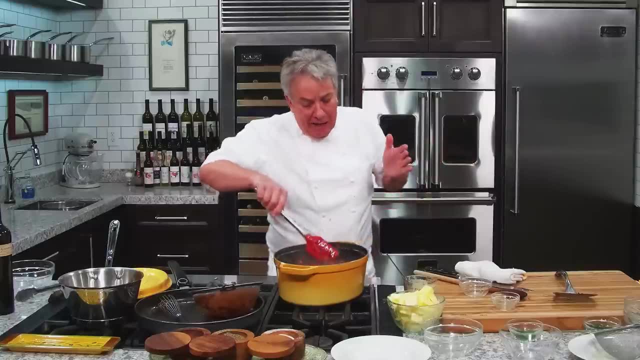 Little little, Not like blub, blub, blub, blub, blub. You know, If you boil it too much you'll reduce it, It'll attach in the bottom. If you do it gently, you know, every so often. just go by and here we go. 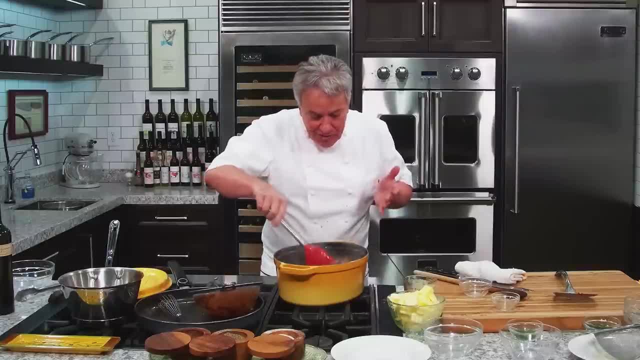 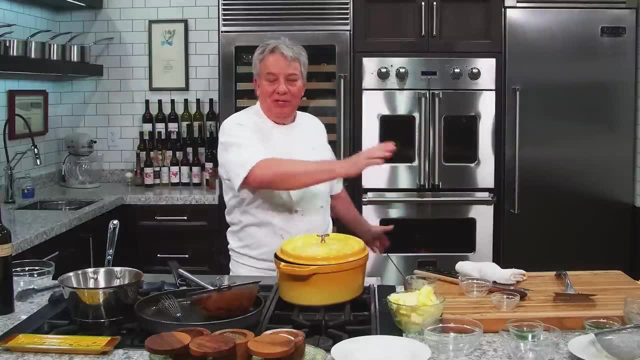 Mix it up a little bit, You know, check it up, Make sure it's good. That's all All you got to do. put the cover back on. You don't have to worry about it Or pop it in the oven and do the same thing after half hour 45 minutes. 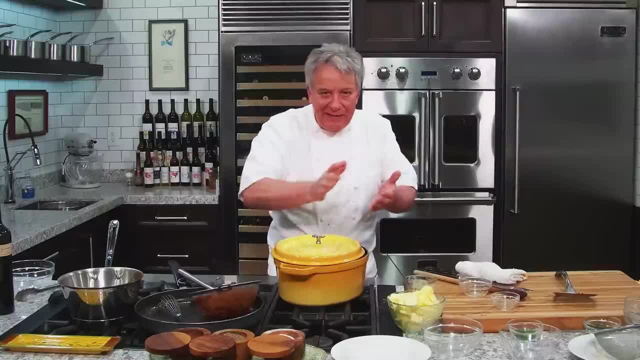 Check it and make sure it's good in the bottom And cook it. two, two and a half hours Depends on the meat you get. It's going to take a little bit longer. It could take three hours, Depends what it is you're using. 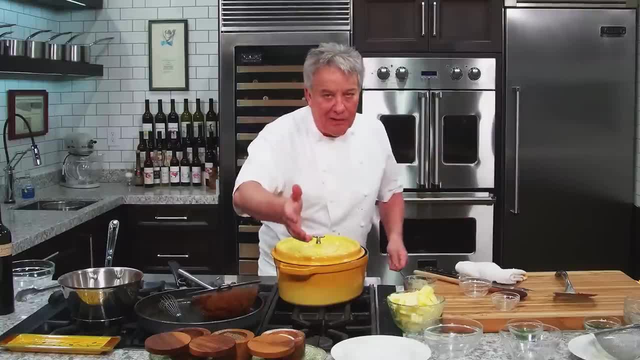 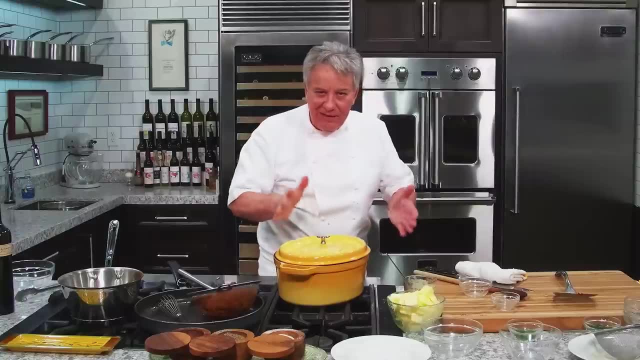 But you got to plan two hours. It's not like you got to work for two hours, You just got to turn it on and go do something and then check it up once in a while, All right. So in two hours we're going to come back and we're going to check and we're going to see how good it is. 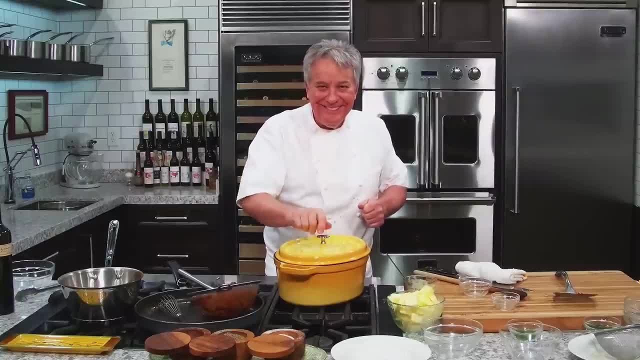 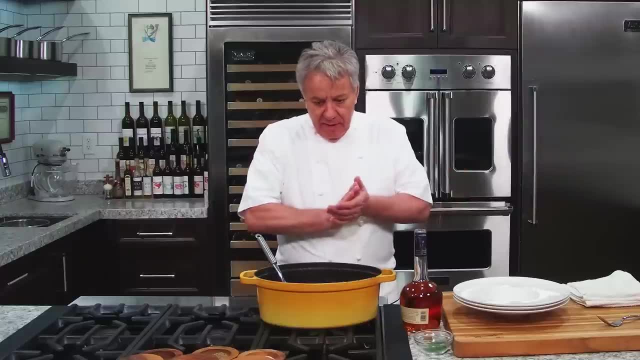 All right, I'll be back in two hours. Don't go anywhere. All right, my friends, What about? two and a half hours went by and we're done, It's finished. I'm going to put a little bit of cognac. 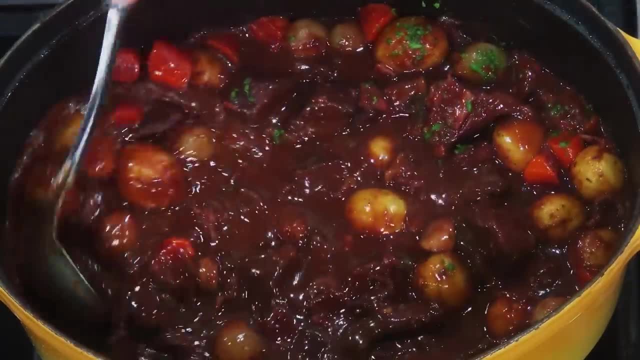 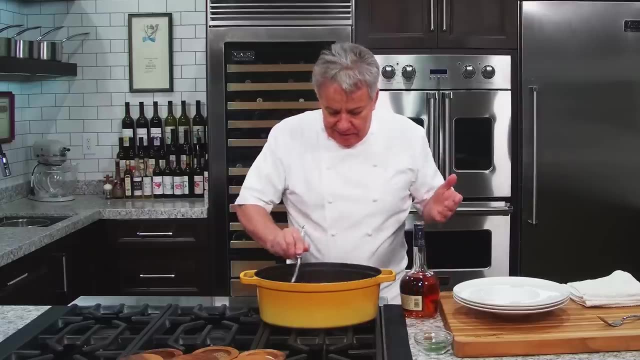 Whenever you put cognac in something, folks, or any kind of booze, really you don't have to put the cognac, Especially for those of you that don't drink, don't worry, Don't need to replace it. You know, some people say: what do I replace it with? 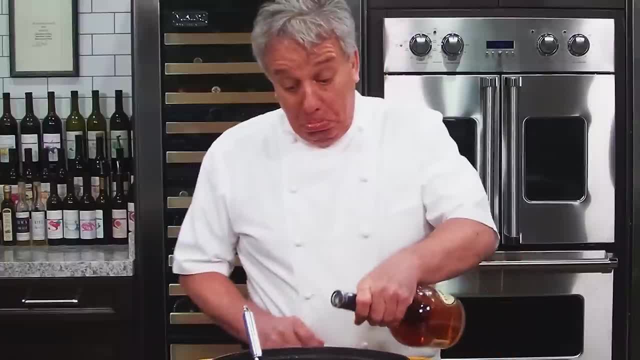 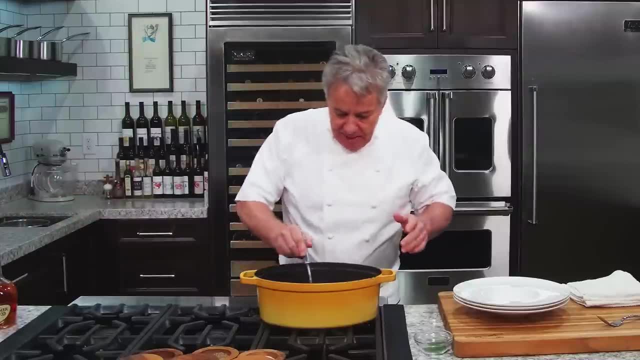 You can't replace it with anything, So don't be afraid to put some. And the reason why I put it at the end is because I want to test it. Otherwise I'm not going to put it in. It makes no sense if I'm not going to test it. 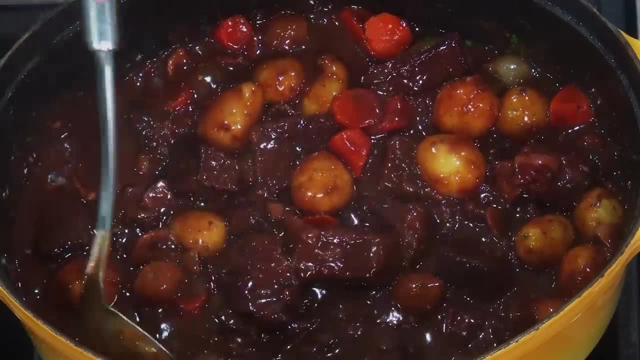 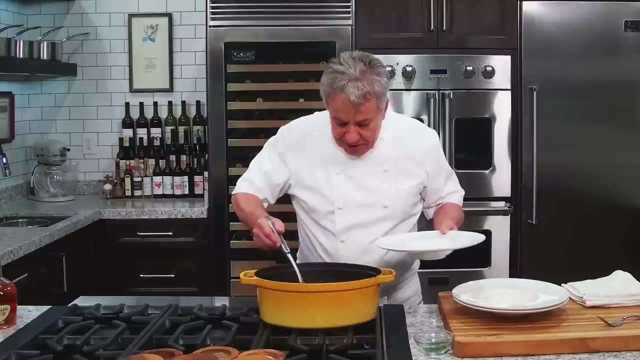 If you put it at the beginning, you won't test it. It's in there, So the meat should kind of fall apart, And the potatoes are cooked, And the carrots are cooked, And everything is cooked And it's done. I mean, this is ah, mamma mia. 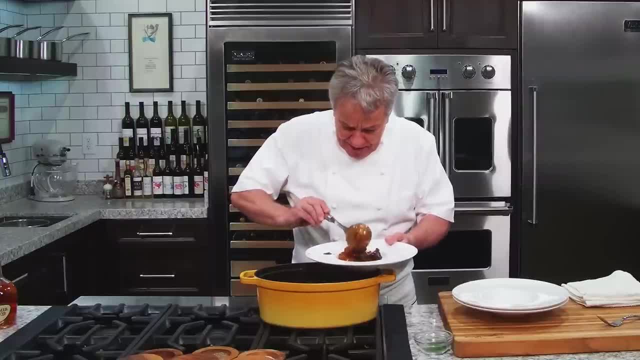 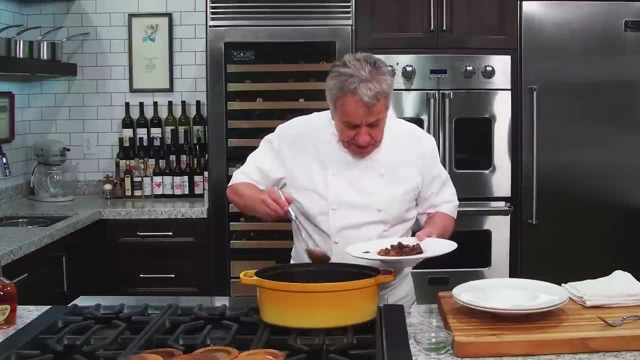 I made a mess, So that's okay, I'm going to clean it up And voila. I mean really, it's really simple, friends. And so you decorate your plate, You put a little potatoes in there, You organize it the best you can, so it looks pretty right. 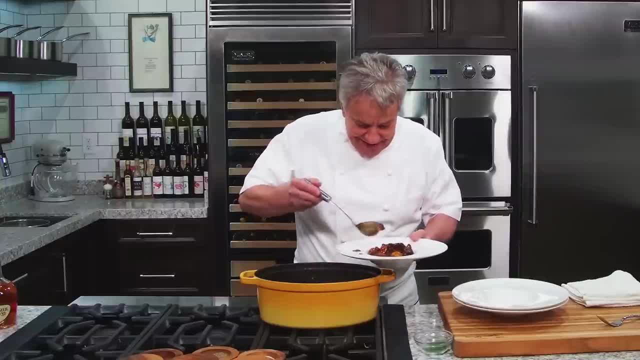 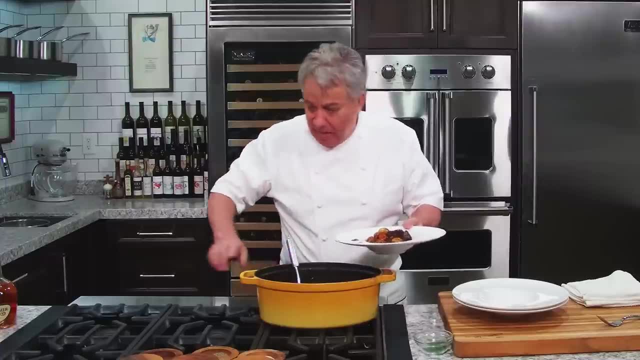 And look at the mess. Don't make a mess like me, eh, Whatever you do- And I put some onion in there, right, So you decorate the plate so it makes it look kind of pretty- Let me get a spatula here so I can clean up my mess. 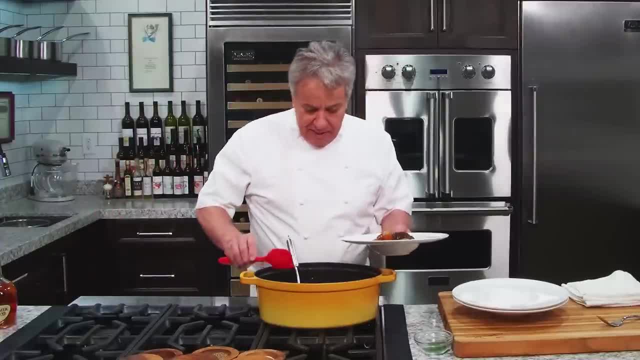 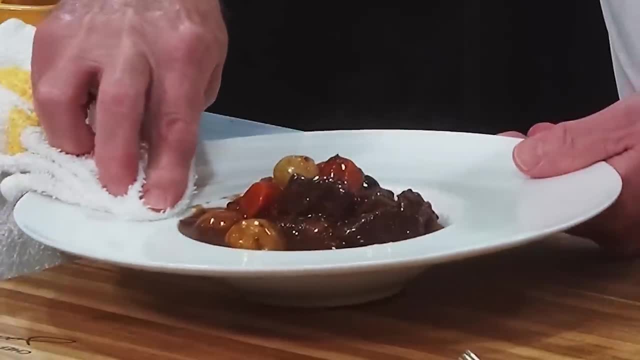 because I hate that mess right there, like that, right And then. so the beauty about, friends, the beauty about is putting the potatoes in there And you don't need to be making mashed potatoes, You don't need to be making a polenta, which will be delicious, right. 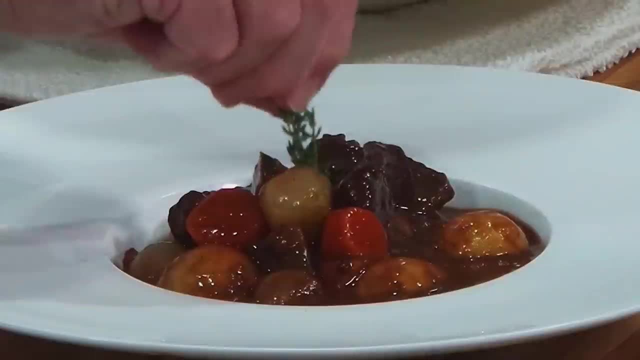 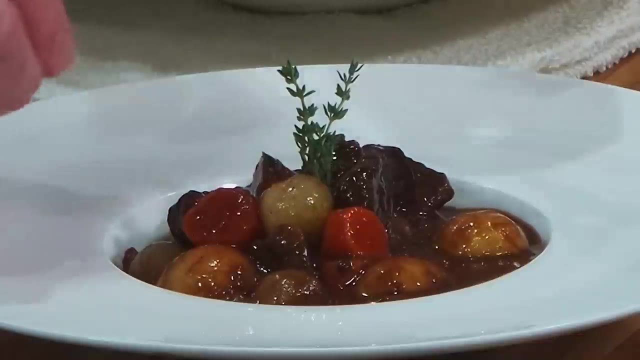 And so remember, we're going to decorate it with a little bit of fresh thyme because that's what we got in there. We got fresh thyme in there, So don't be putting fresh thyme on top of a dish that doesn't have fresh thyme in the dish, right.